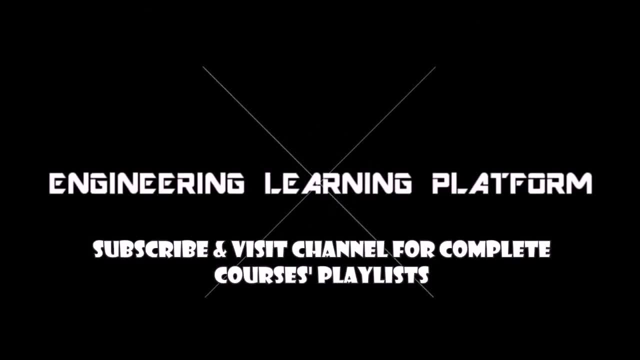 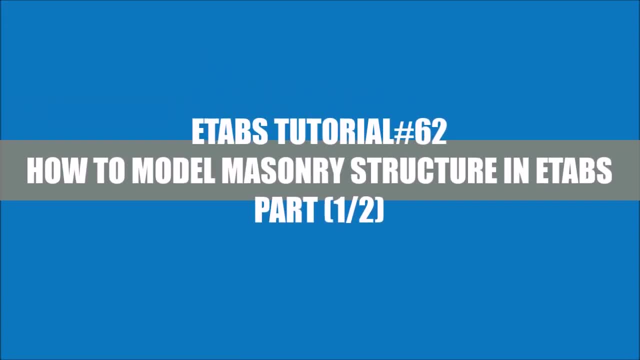 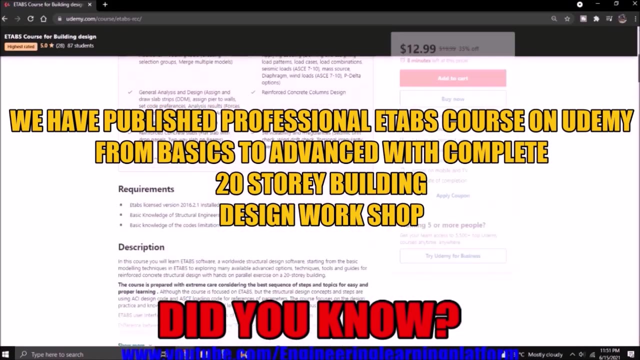 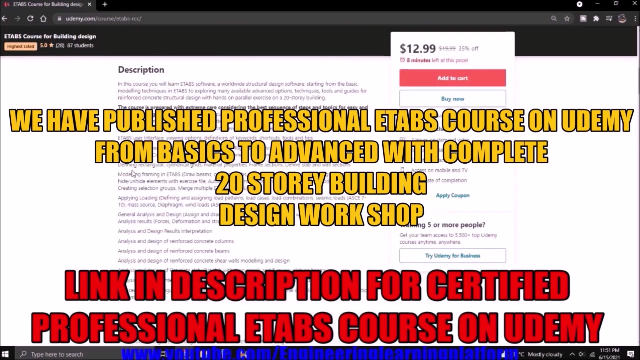 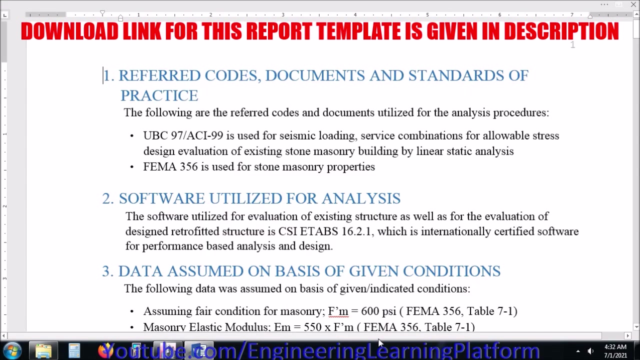 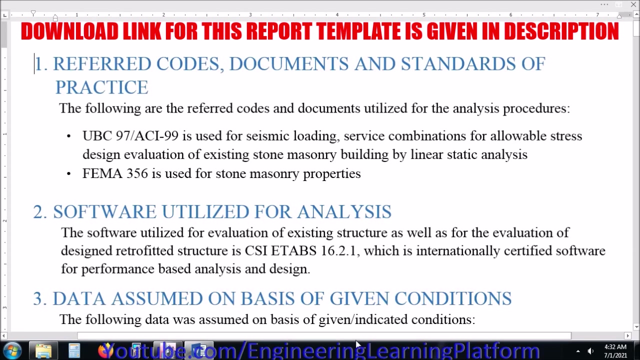 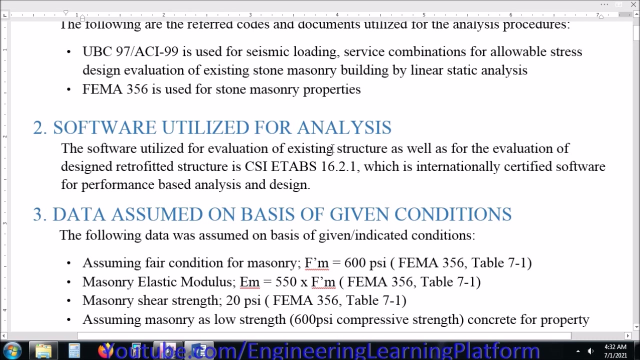 Did you know? We have published an ETABS course with a complete 20-story building design. The course will include complete guide to ETABS, from basics to advanced level, with a completion certificate Check link in description of this video. The software to be utilized will be ETABS, As we all know that we are using the ETABS 2016,, which is the most stable version of ETABS, till the publishing date of this video. 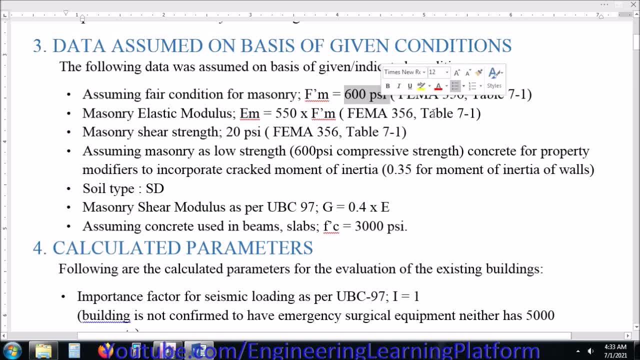 I am assuming fair condition masonry ie 600 psi compressive strength. the preference is given, the modulus of elasticity of the masonry is also given and the reference is given. The strength is 20 psi. again along with the reference from the FIMA 356 table. 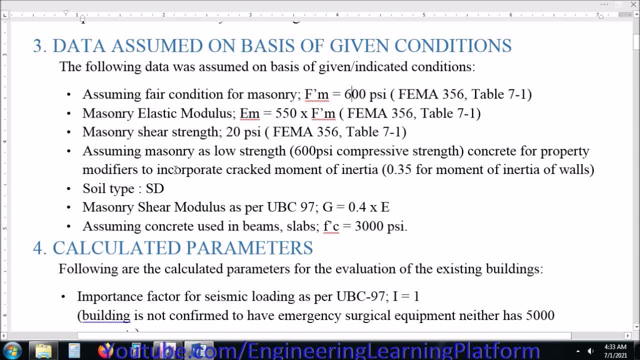 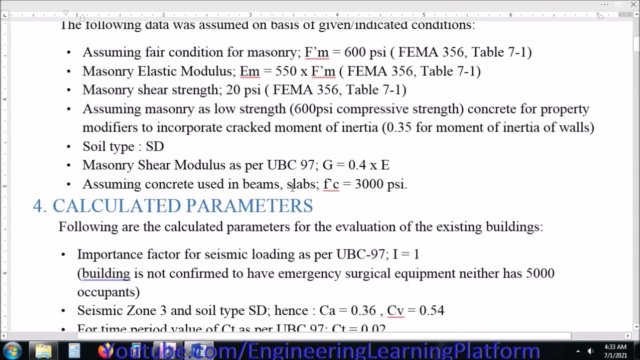 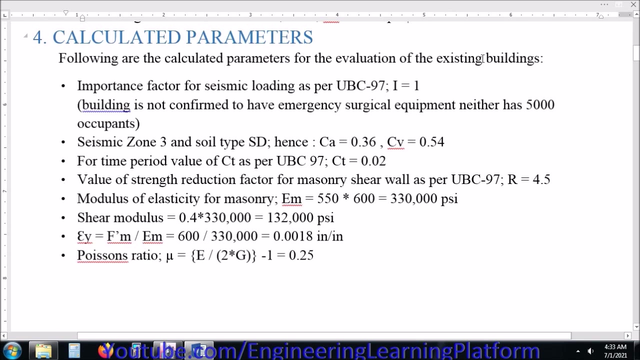 I am assuming a low strength stone masonry and the modifiers will be incorporated for the concrete as 0.35 for moment of inertia of the walls. We will be taking the soil type as SD. Seismic parameters and other parameters are also discussed in detail in that document. 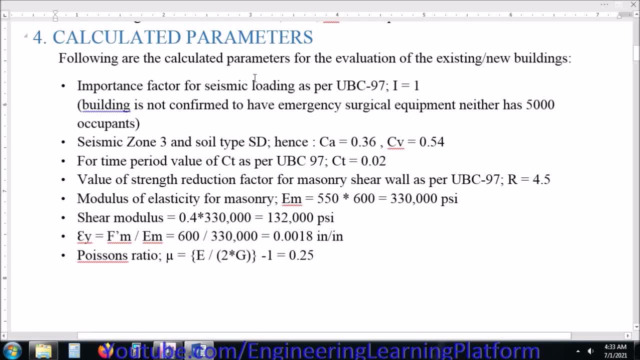 We will be starting with the importance factor for seismic loading. The building is confirmed to have emergency equipment or it doesn't have 500,000 augments, So the importance factor will be 1.. Seismic zone 3, soil type SD. 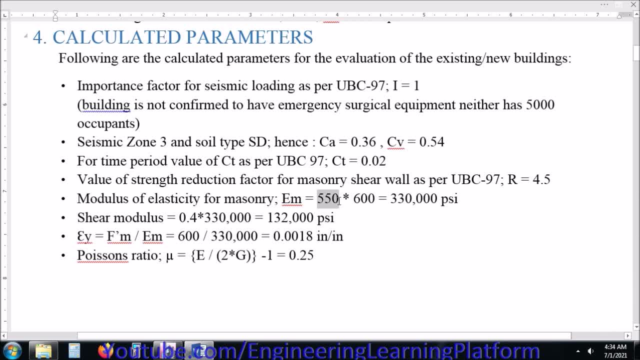 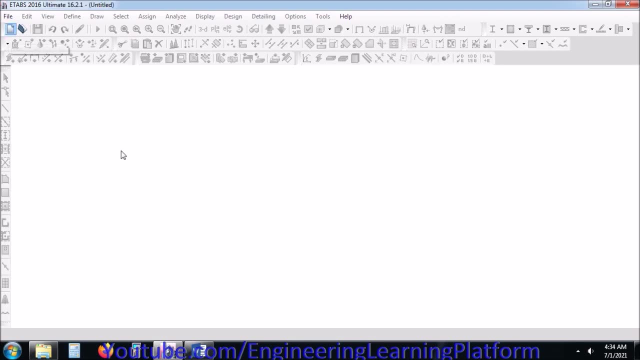 So we are getting the seismic coefficients. You can also edit this report for your design code requirements. It's easily editable. However, the template is highly useful for the report format of the masonry structure, design or analysis, And highly acceptable as I have utilized personally in many projects. 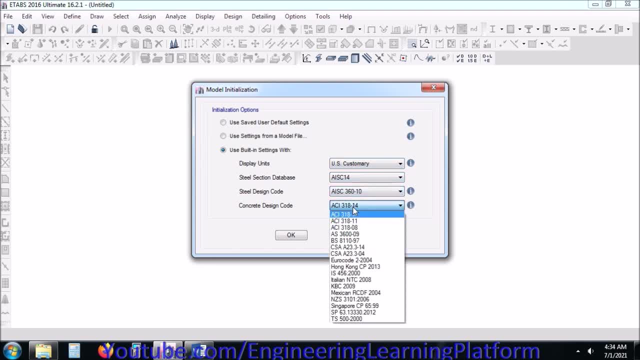 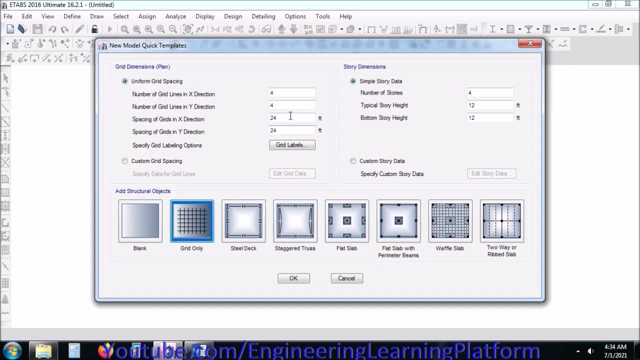 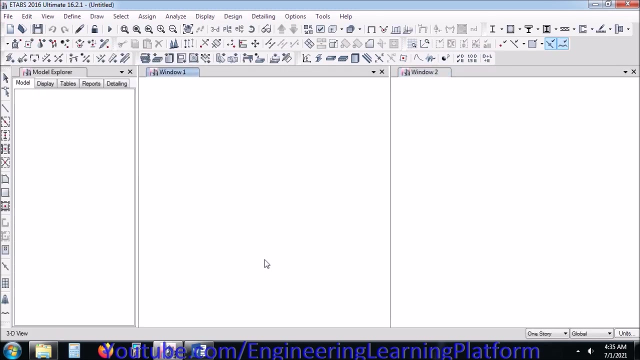 So I will be defining the grids first. So I will be defining the grids first. Let's take it as 20 feet in X and Y direction. Number of stories is 1. since it's a one story structure, I'll be adding the new material. 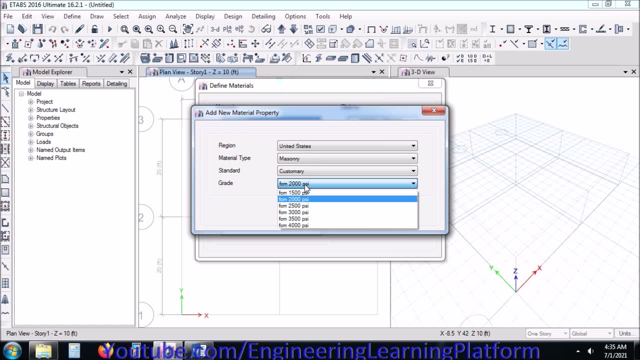 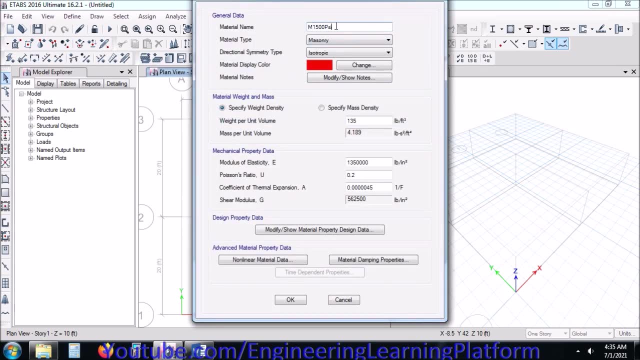 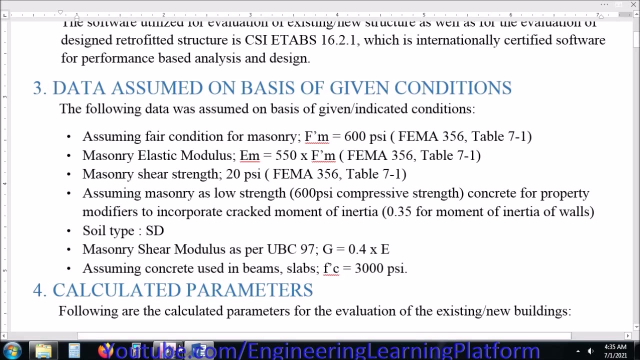 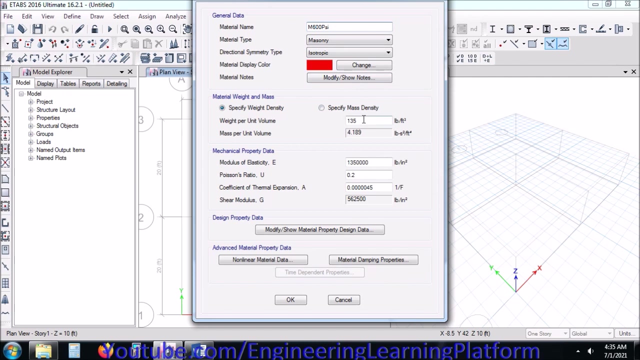 ETABS has built in masonry option and the FC we are to be using is 600 PSI, but the minimum is specified here is 1500 PSI, So I'll be editing it to our material. that is 600 PSI. compressive strength: The density remains same. 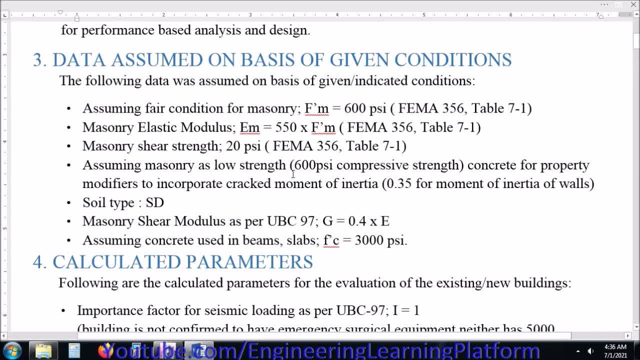 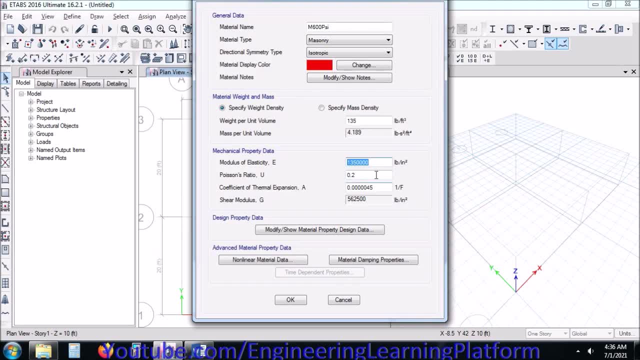 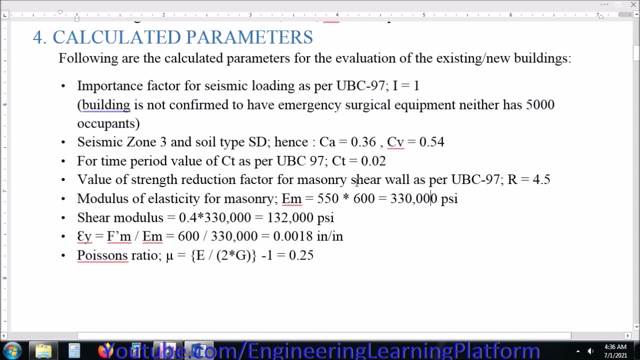 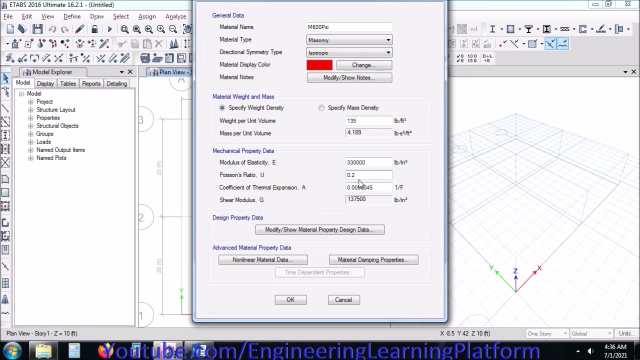 We'll be checking this property from the table. We'll calculate it: 550 of the formula into 600, that is the compressive strength, We get a value of 132 or 330 PSI And the Poisson's ratio is 0.25, as we'll be observing the stress in the material induced. 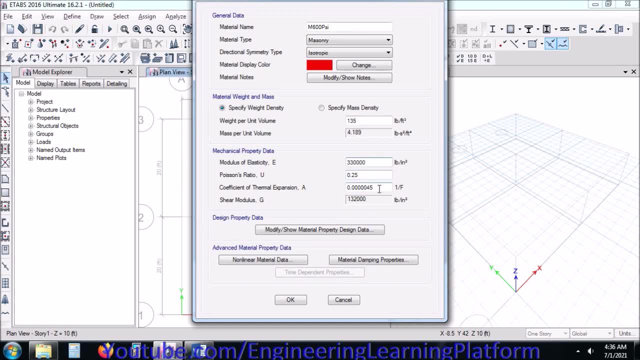 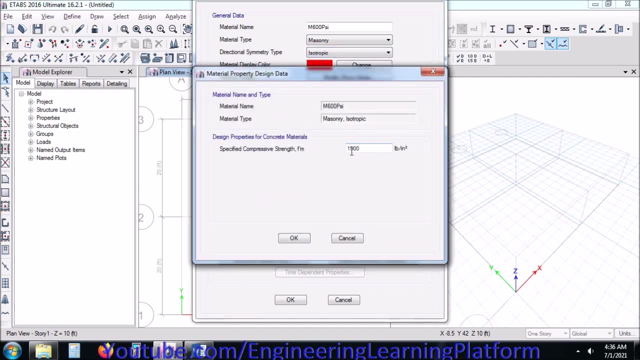 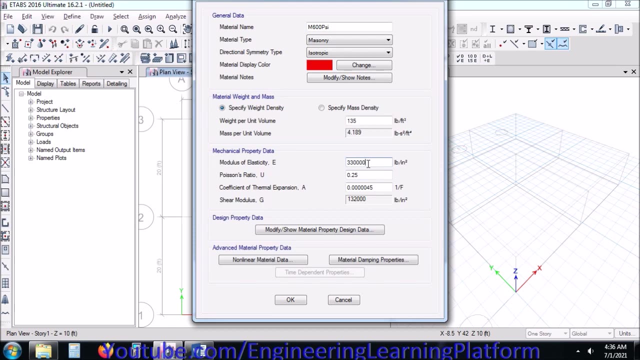 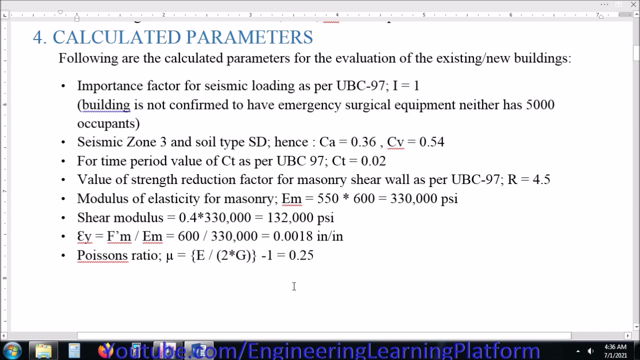 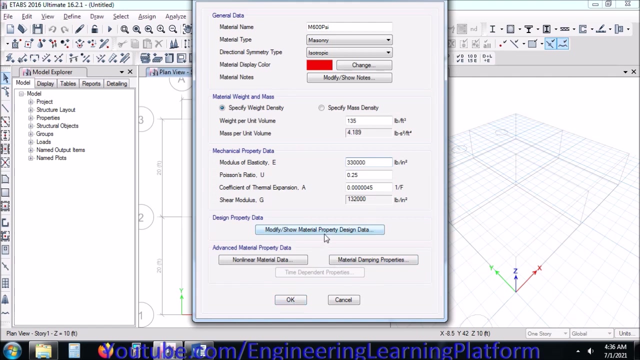 by the loading. So these properties are highly important, Even for linear stress And static analysis. Let's modify the compressive strength property of the material, that is 600 PSI bounce per square inch, And then click on OK. And then click on OK. 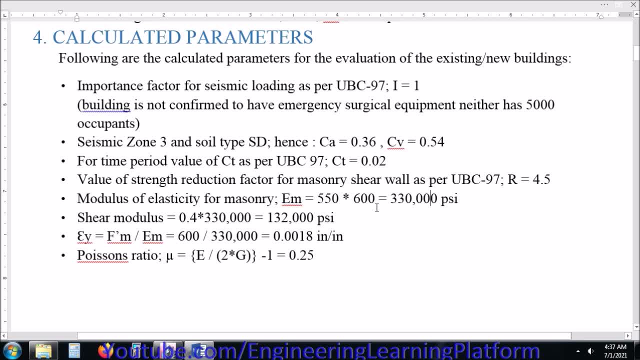 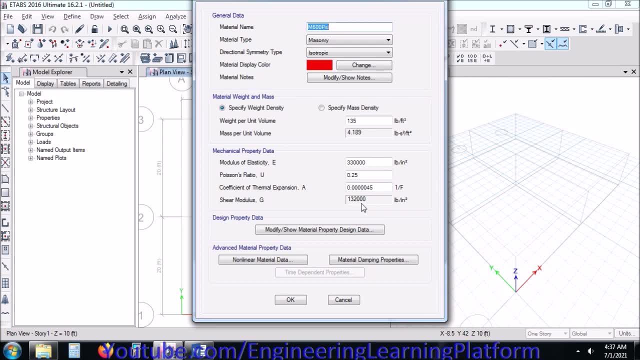 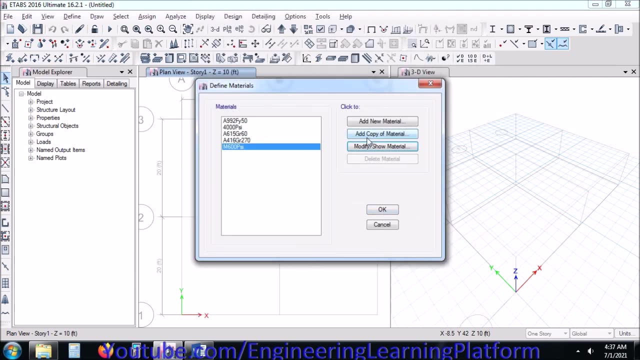 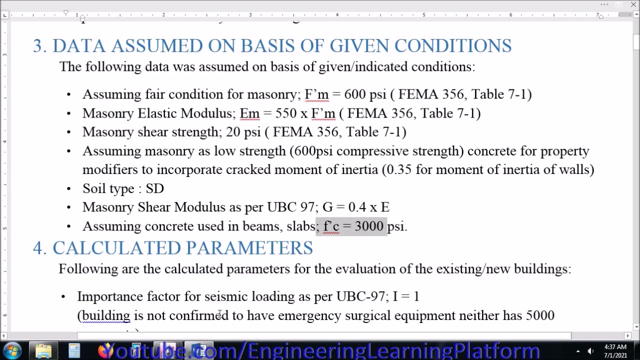 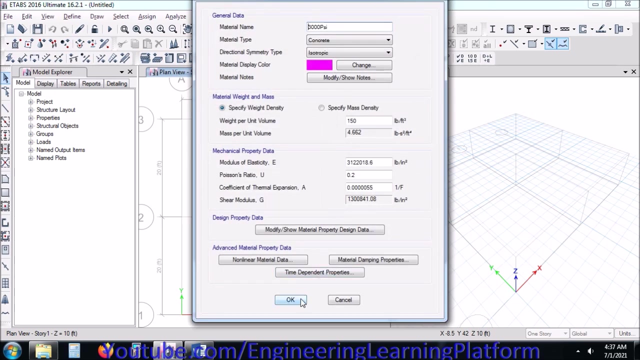 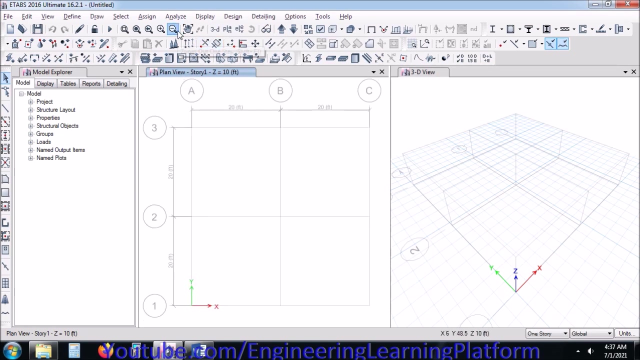 Let's take a look: The compressive strength of the concrete. since we will be using the band beams, the reinforced edges, it would not be right to call them as columns, as there would be two slender and small sections, so I will be calling them as reinforced. 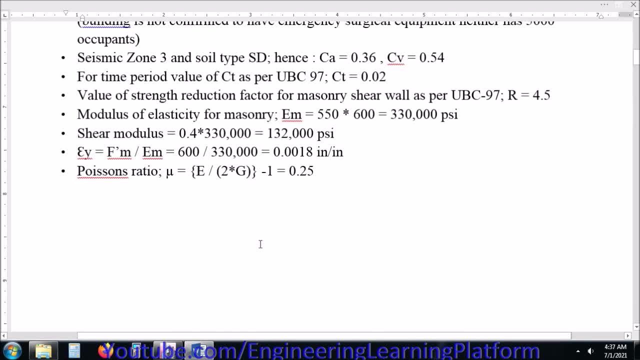 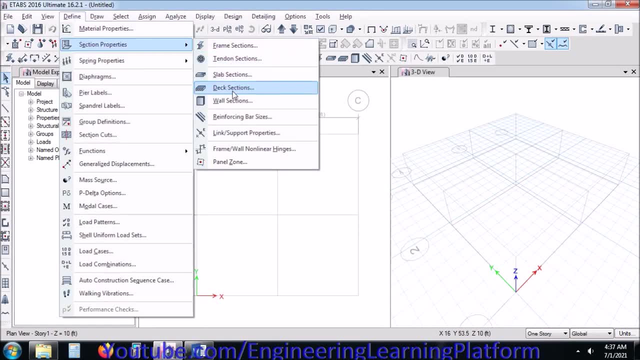 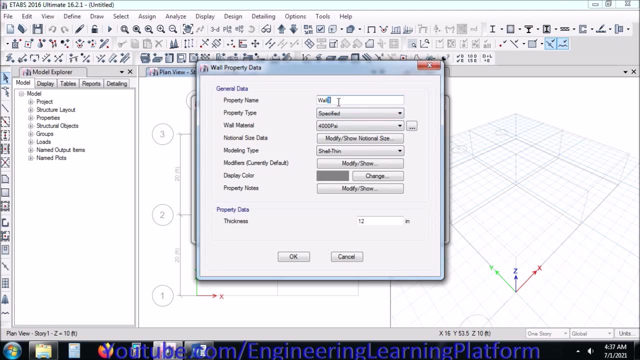 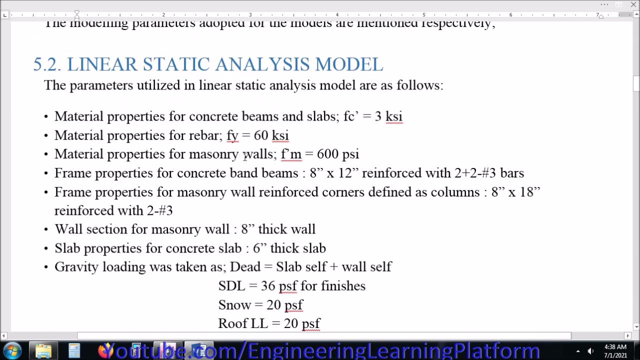 edges of the wall or reinforced interlinks between the walls, as it may be required that we will be providing these reinforced corners or portions of the wall in midway of the wall. so let's define the wall section of the masonry. the masonry wall we are thinking to take is starting with 8. 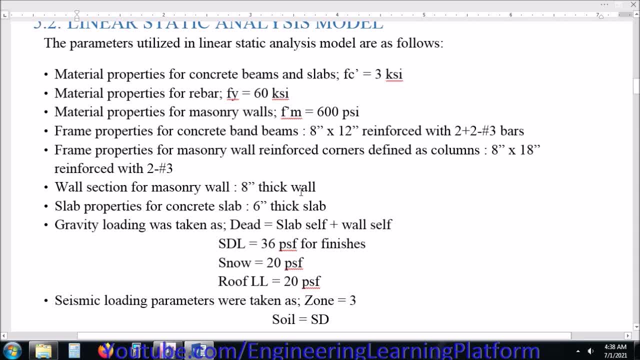 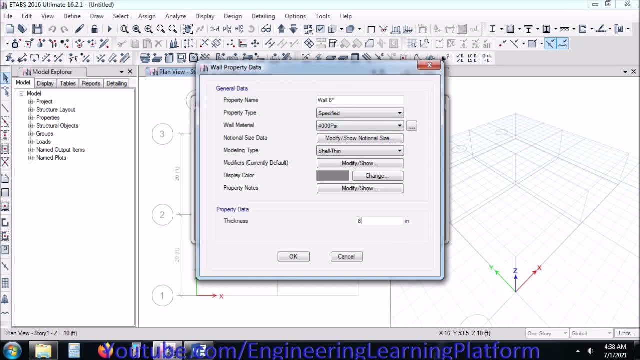 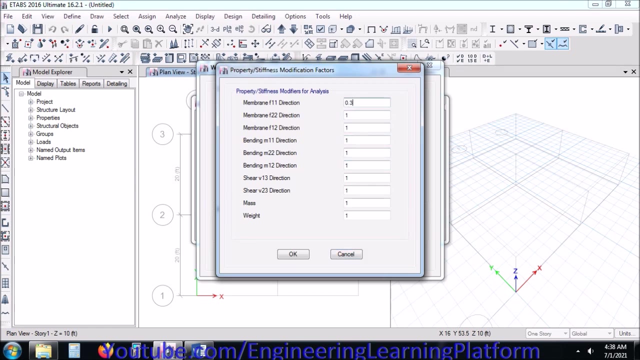 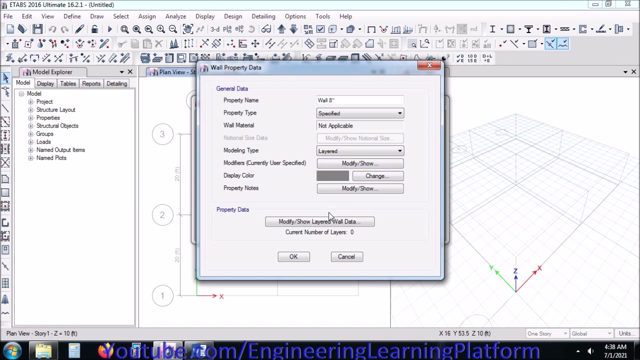 inches, as the block size is of 8 inches we will be using in the project. usually it is also specified that the thickness is to be taken by the architect, so I'll be using the 8 inches thick wall. so I'll be taking crack moment of inertia for the walls because the 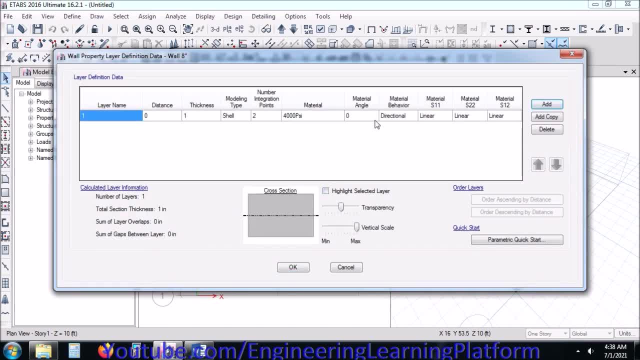 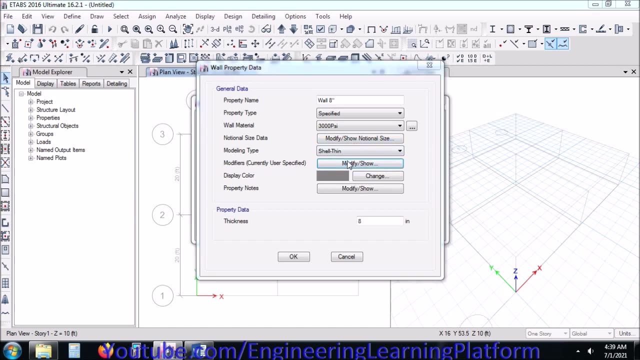 reinforcement provided in the walls will be just at the defined edges. we can also take the properties as layered, but it would be too complicated for the analysis. rather, we'll stick to the simplicity and go with the simple wall with a uniform cross-section and then click on OK. 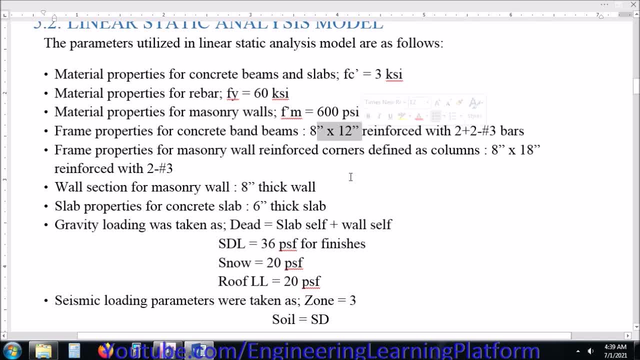 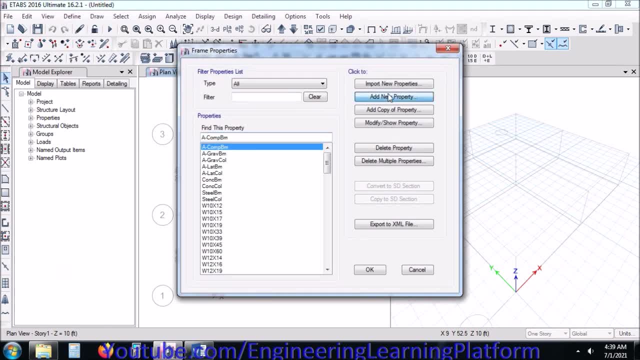 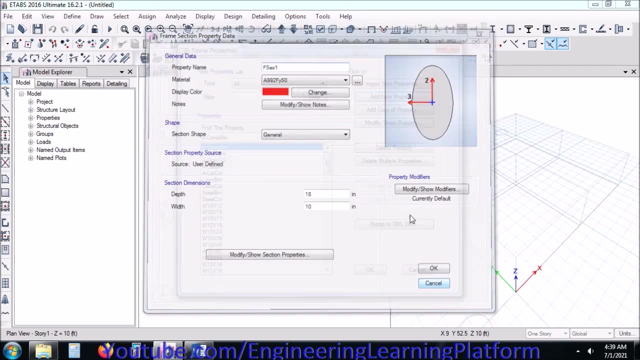 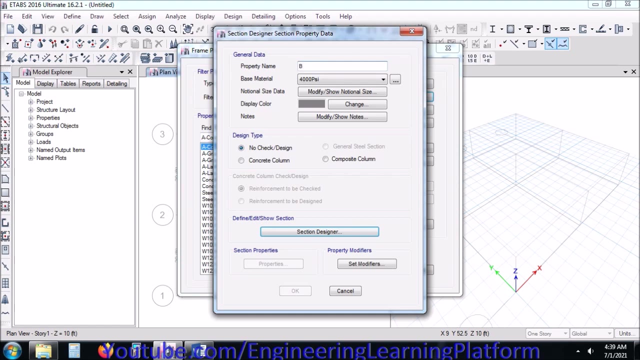 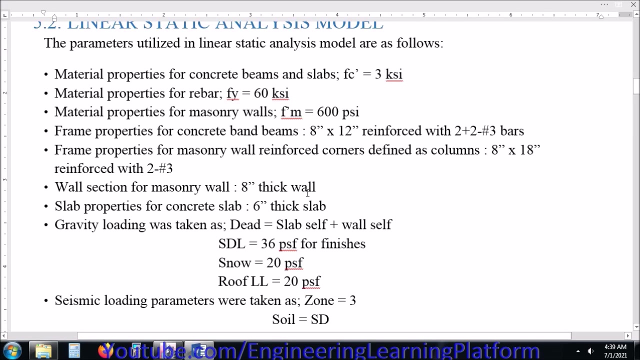 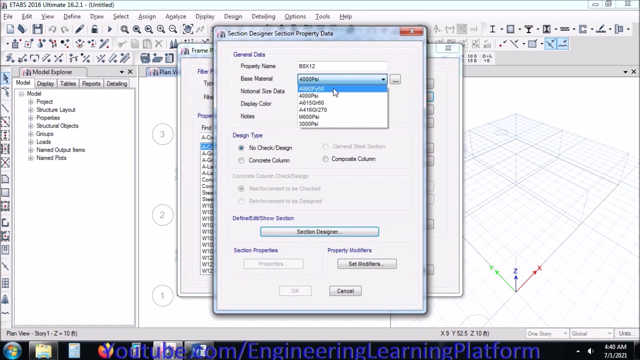 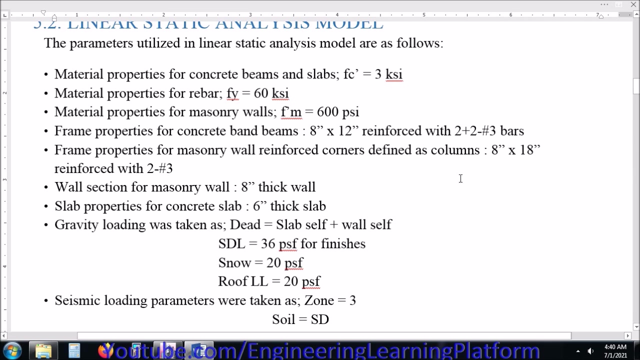 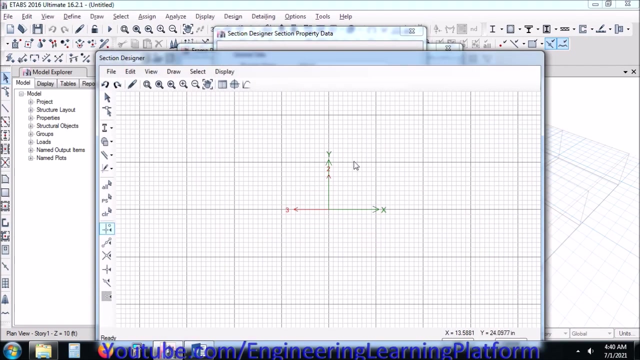 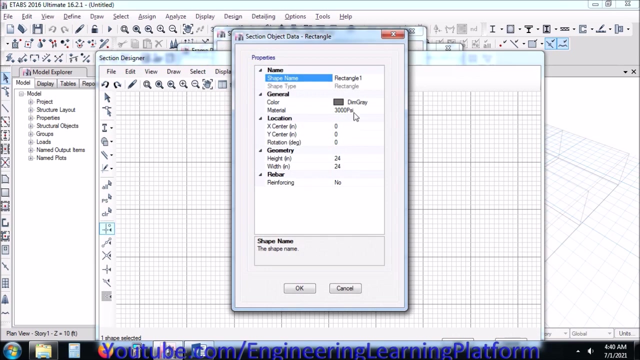 frame properties for the band beams to be defined is 8 inches by 12 inches. let's go to define section properties and frame sections 8 by 12 inches, and then the wall section for all the ready. now I'll be taking the reinforced edge of the wall, so i'll be taking the 3000 psi concrete for this particular area. 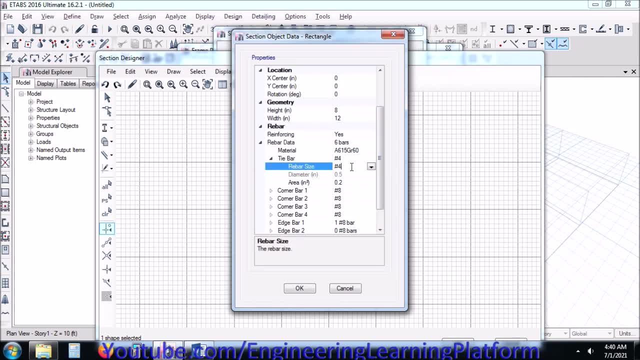 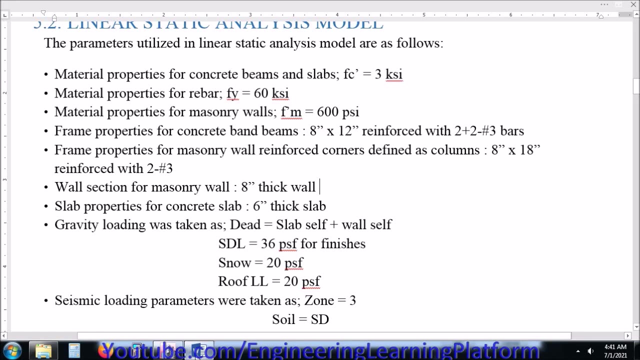 if you are using hollow block, you can simply enter the compressive strength of the block, but i am using the concrete edges of 3000 psi, so i'll be using the compressive strength of the concrete. you can enter the corner bar, information and the other information. 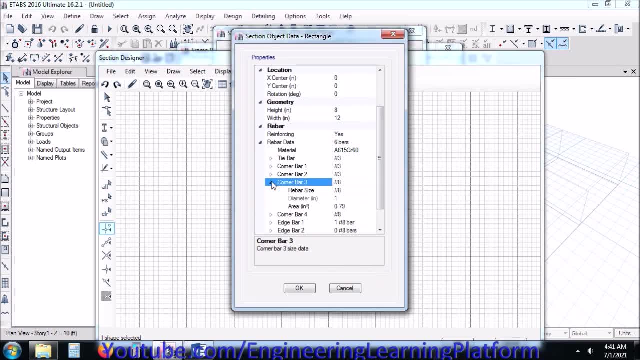 similarly for the bank beams. i am taking the compressive strength of the concrete, since the band beams are of reinforced concrete. i am specifying the number of bars, since we have only corner bars, so edge bars are being set to zero. actually, we have to rotate it, so 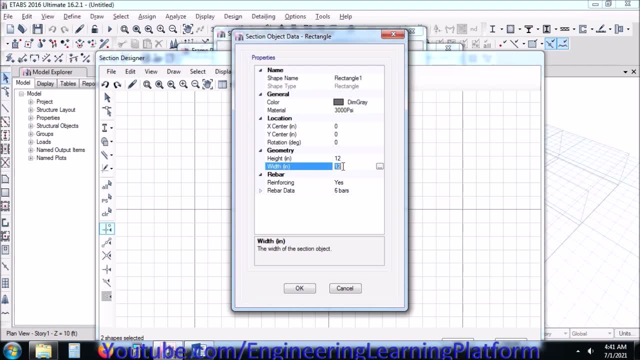 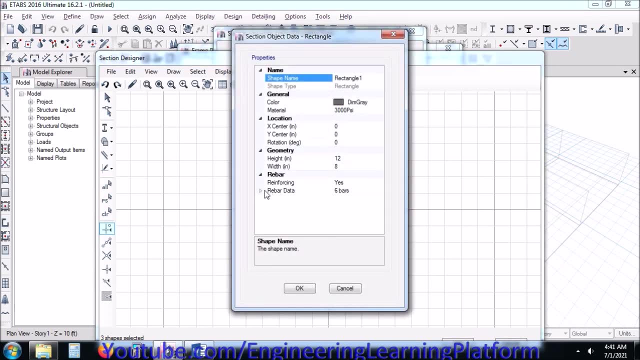 make this one 12 and make this one as 8 inches. now it seems fine. oh so we have two extra bars, so i'll be removing these bars. we already made the edge bar zero, but once we rotate the shape, it again resets the bar at the particular edges. 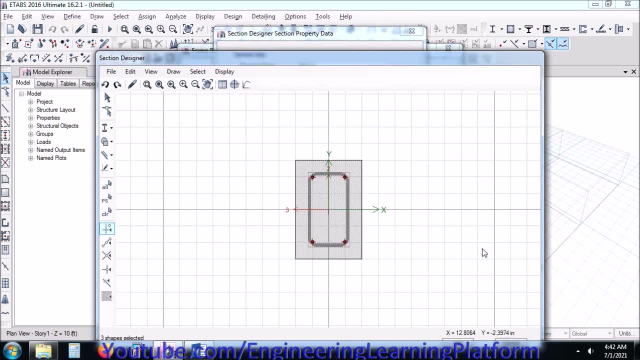 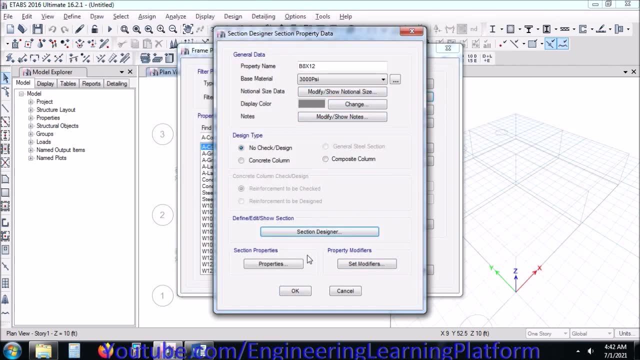 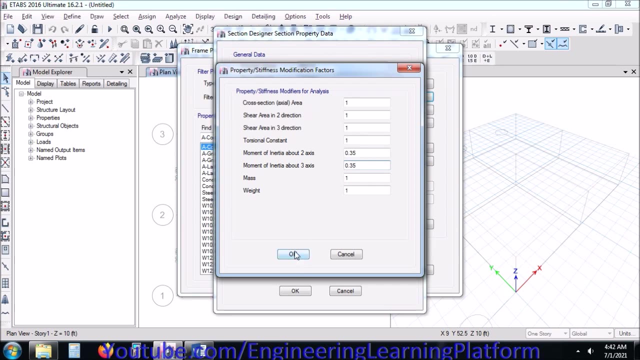 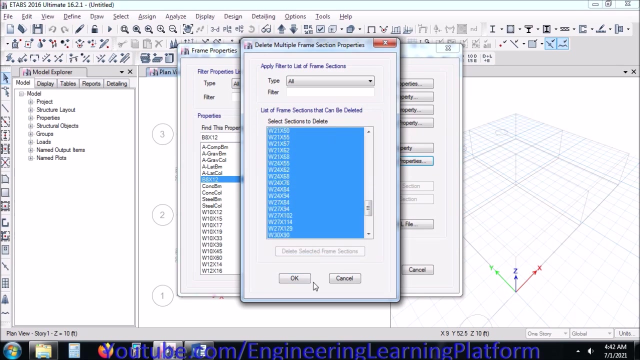 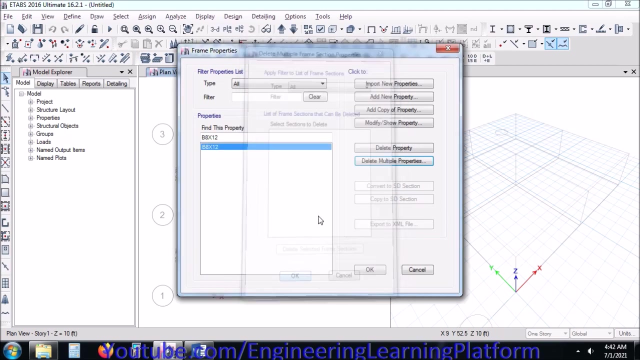 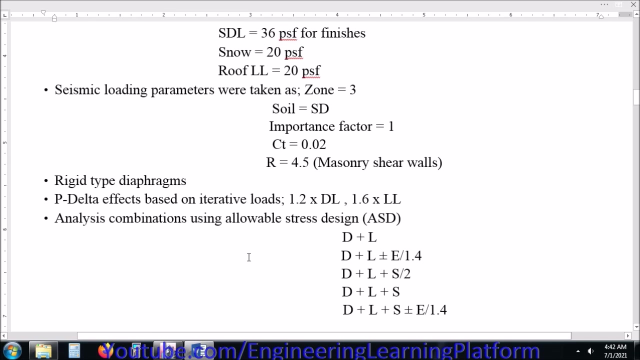 and click on ok. similarly, click on ok here and here. let me just save my entire connection for the moment of inertia so you can set the property modifiers for the beam here as per ACI code to incorporate the cracking of the moment of inertia. click on ok. now let's define the column section or the reinforced edge, the. 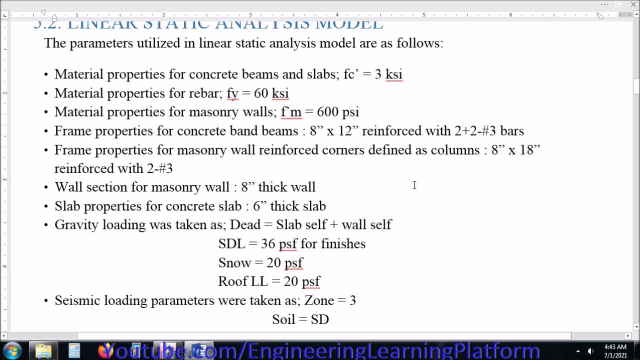 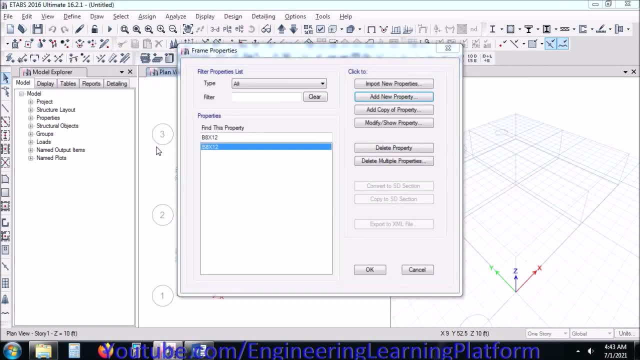 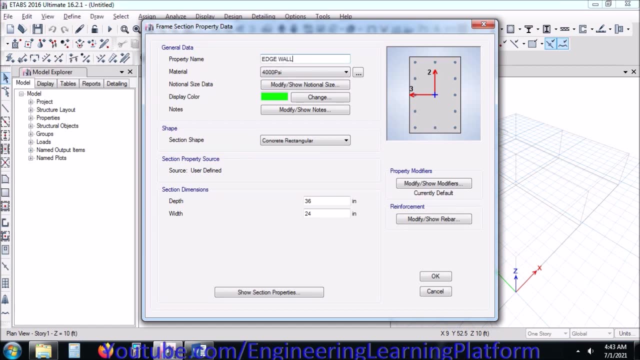 section size is 8 inches by 18 inches in force, with two number three bars. I don't think I can place two number three bars in section designer. even so, I'll be placing four number three bars, as two number three bars would be too short for. 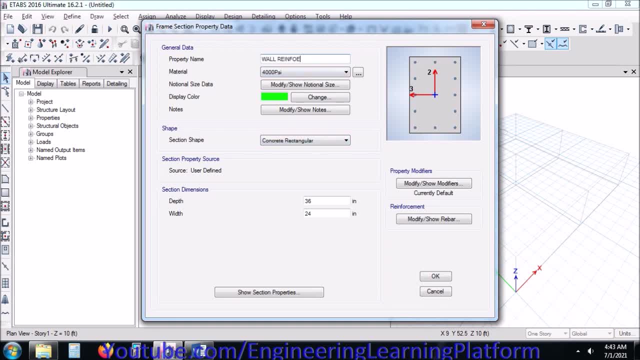 an 8 inches wall. I'll repeat again: if you are using the reinforced edge for the hollow block masonry, then you can take the material property as masonries only, but still I am using the concrete edges of the wall, so I will be sticking to the concrete property. now the moment of inertia. 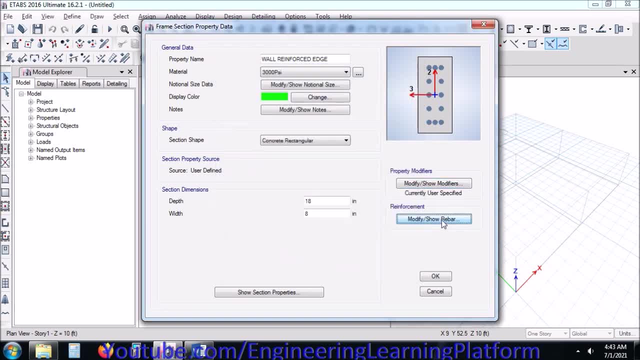 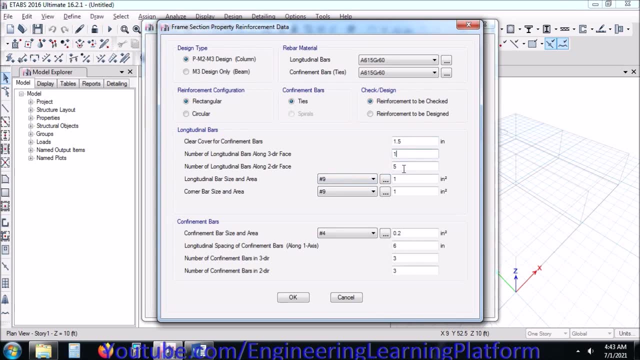 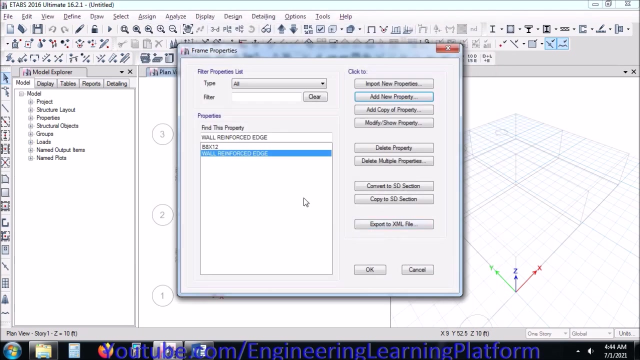 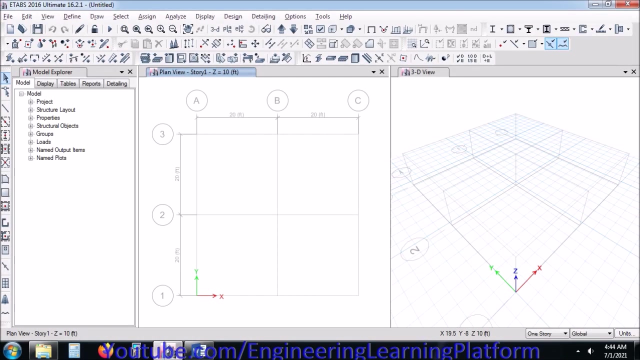 For the edges or the column shape member or the vertical reinforced member is 0.7.. I'll click on reinforcement to be checked and then define the reinforcement. We are having a 6 inches thick slab. Let's modify the slab property, Ok. 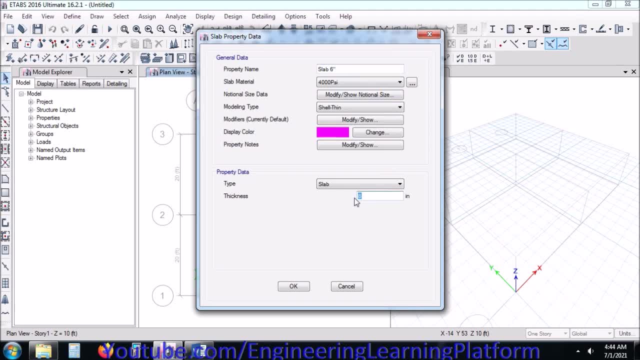 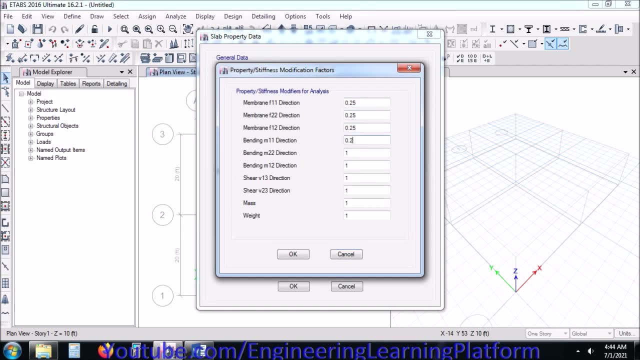 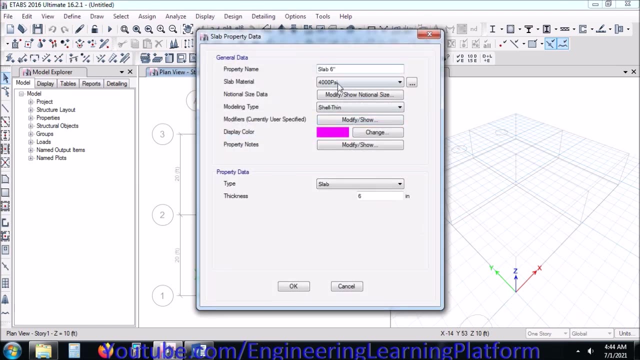 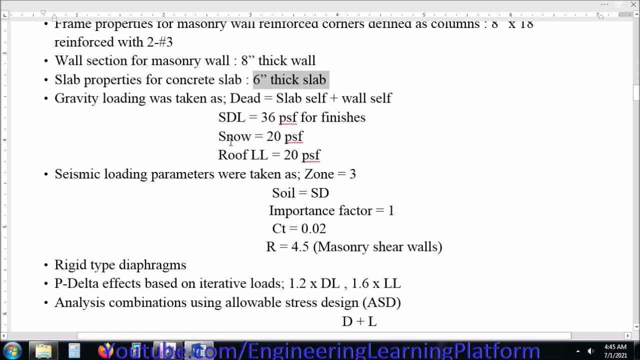 And the property modifiers for the slab, The property modifiers to incorporate the cracking of moment of inertia according to ACI code, And click on ok. You can use these modifiers and other properties as per the code you are using. However, the basic concept remains same. 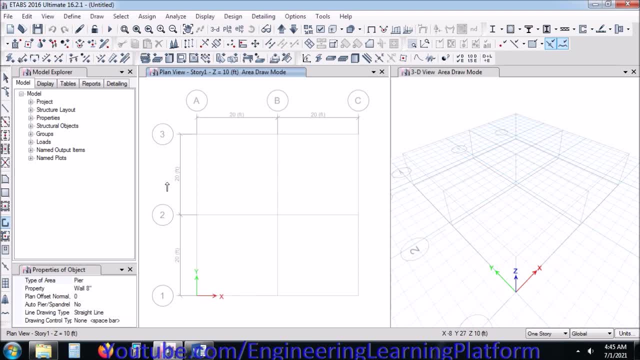 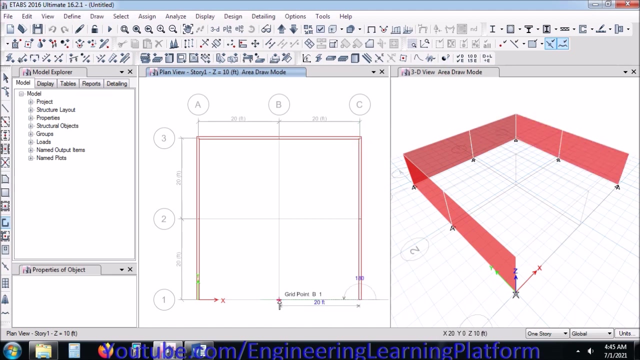 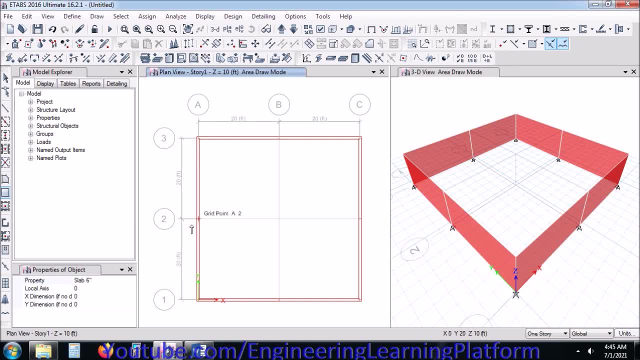 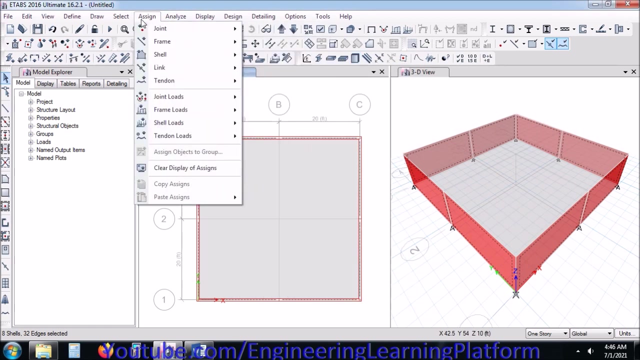 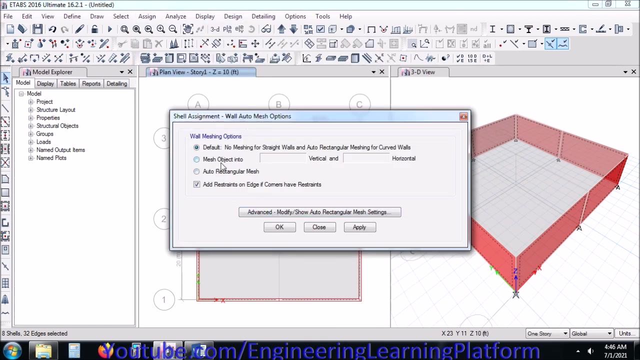 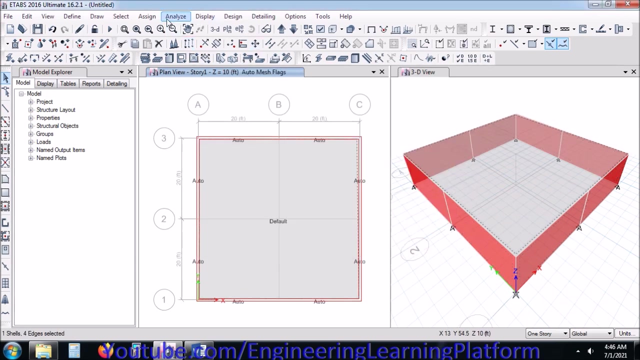 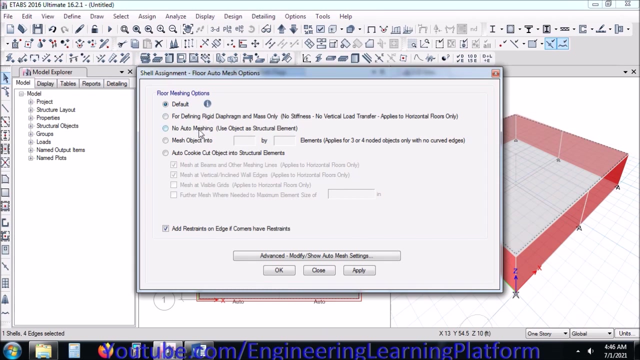 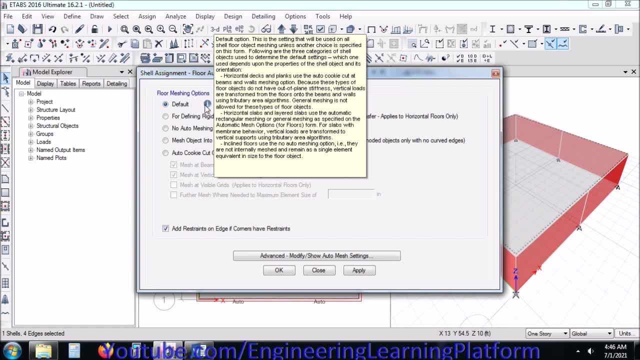 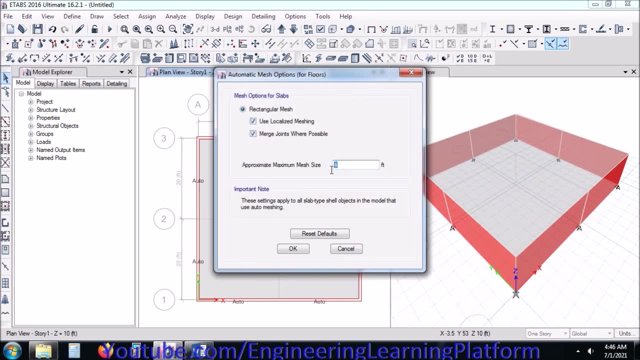 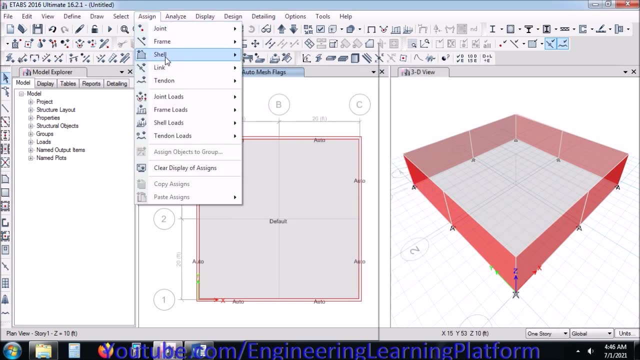 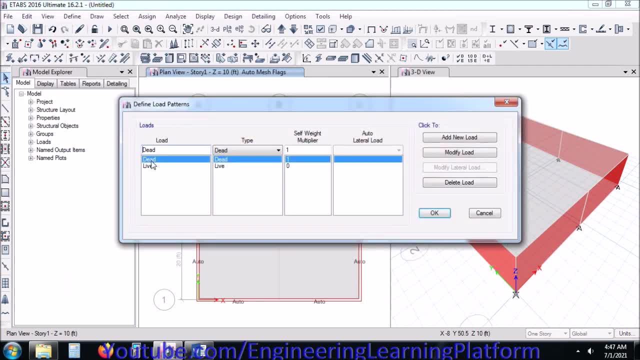 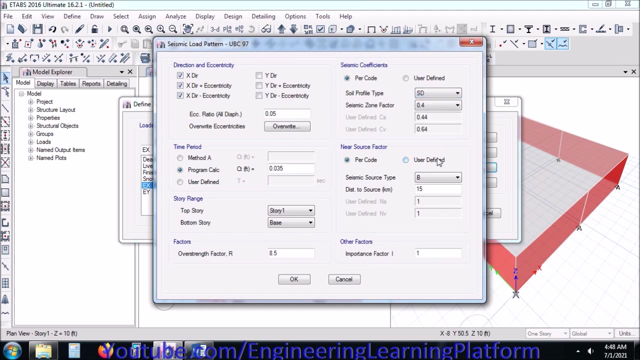 analysis. you dead. live snow and super dead. similarly, earthquake in X direction. that is seismic load. according to UBC 97, you can define the earthquake in any respective code. in a similar manner, you define it for reinforced concrete structure. let's uncheck the y-directional forces and select SD, that is the soil type given to us and seismic. 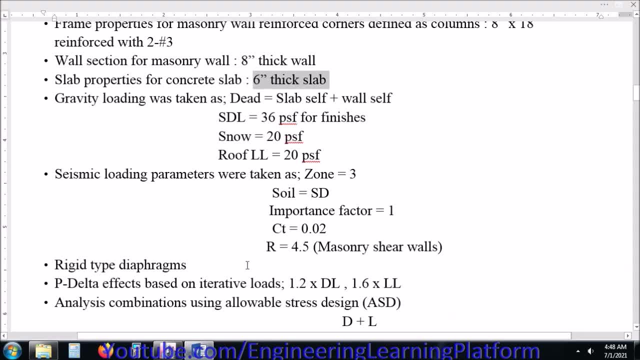 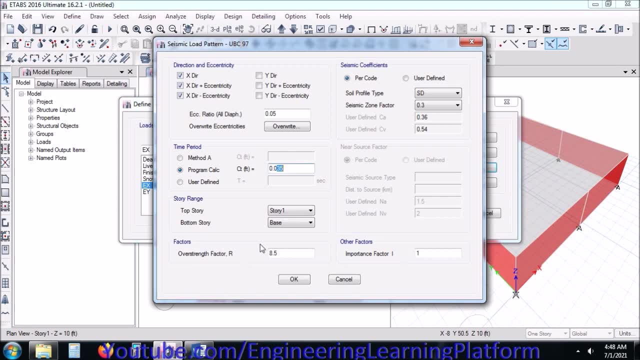 zone 3 the program. so the CT value for the messenese structure is 0.02s and the strength reduction vector is 4.5. so incorporate the ductility of the structure. these all parameters were defined as per UBC 97. you can. 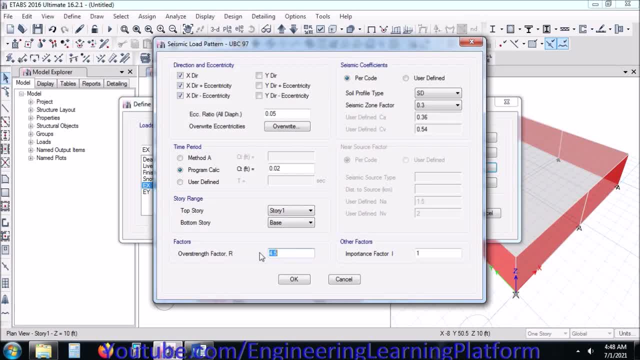 incorporate these factors for your respective chords and sensors. as i selected ubc 97, so i will be incorporating the perimeters in ubc 97 format. so i will tap sd and seismic zone 3 over strength factor 4.5 and click on ok and ok from here to exit. 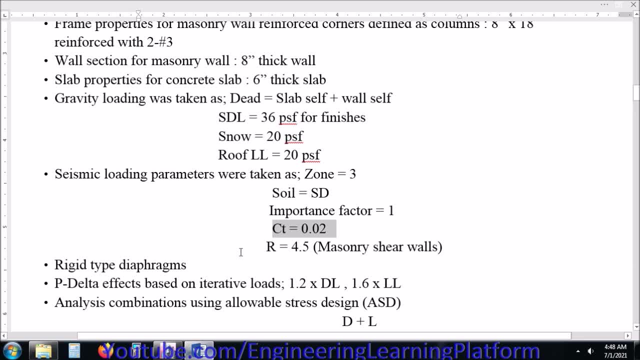 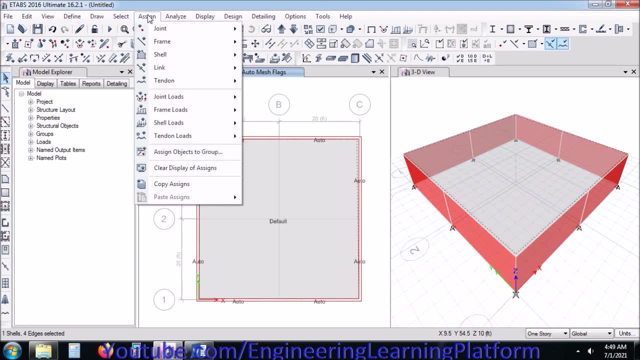 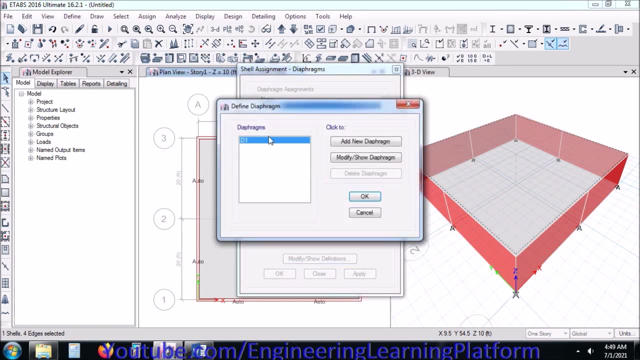 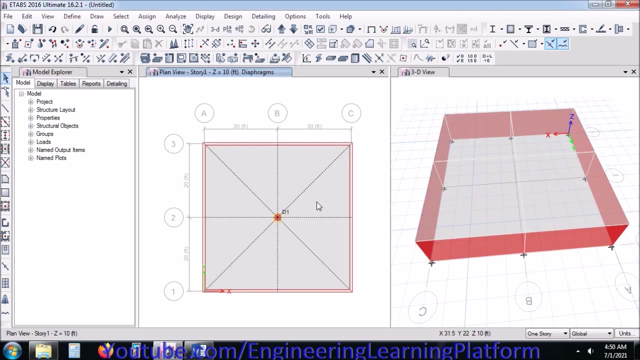 the menu. now. we have defined all the loads. now it's time to apply the loads to the structure. assign the rigid type diaphragm to the slab, so the diaphragm lies in the center as the structure is symmetric, so it means the modeling is done correctly. 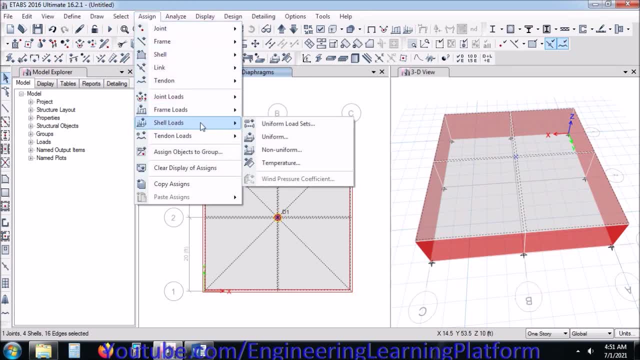 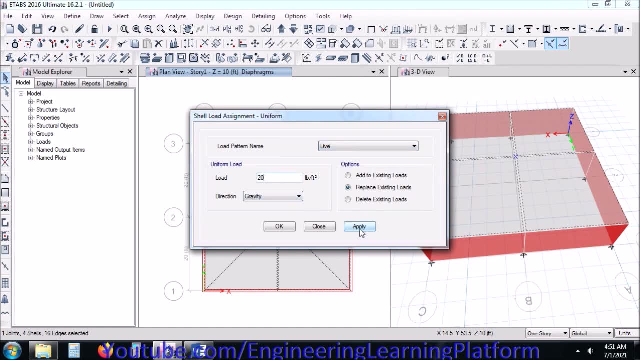 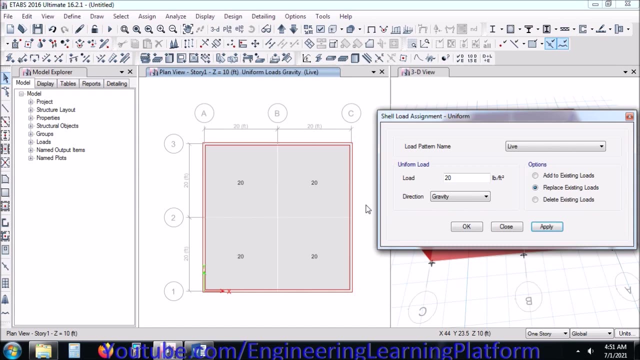 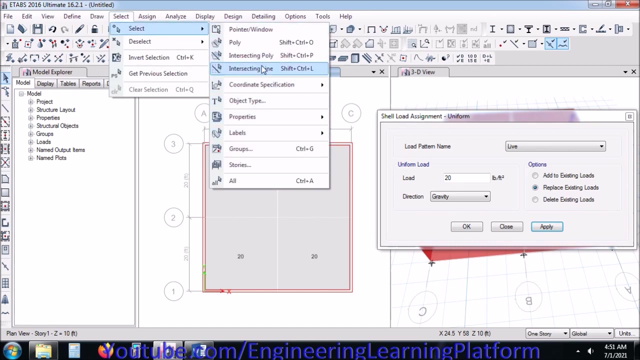 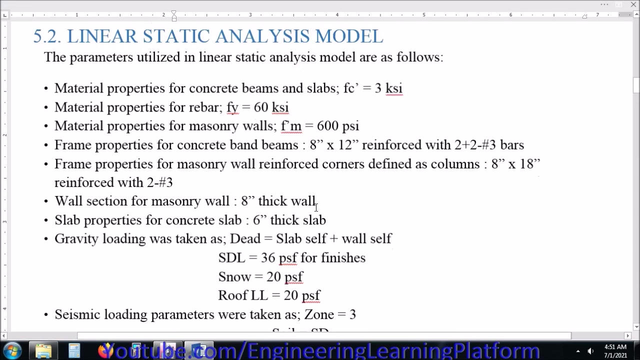 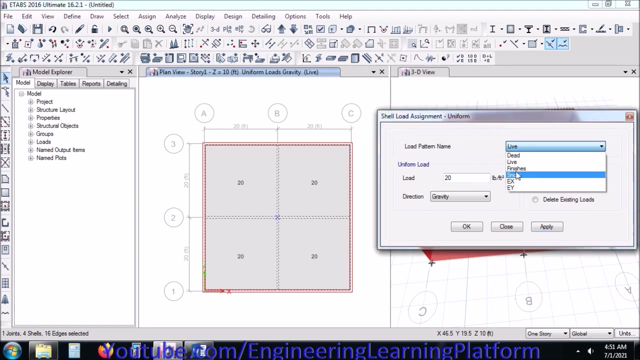 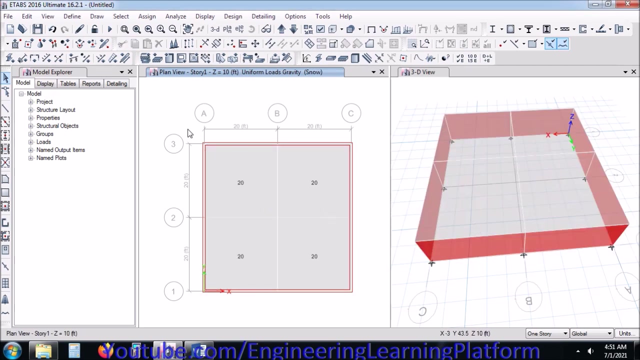 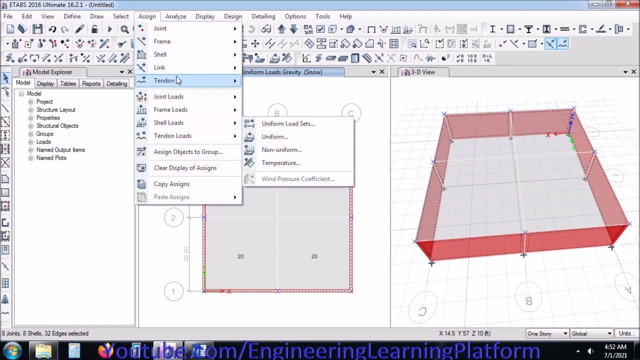 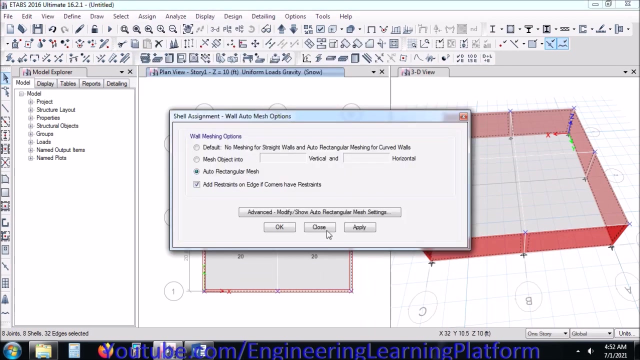 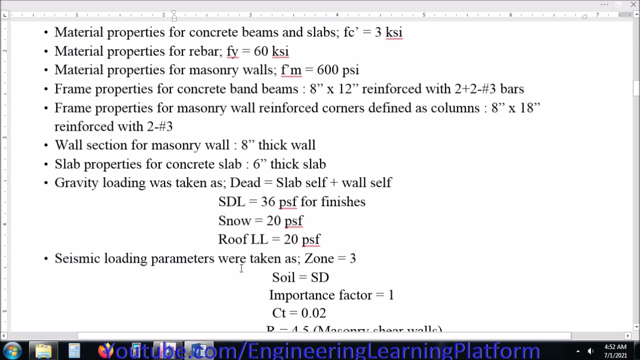 so assigning the live load to the roof and similarly I'll be assigning the snow load and the finishes load. the super dead load for the finishes is 36 pounds per square feet. similarly, the snow load is 20 psf. so mashing the wall, as we previously assigned, in two feet maximum size to 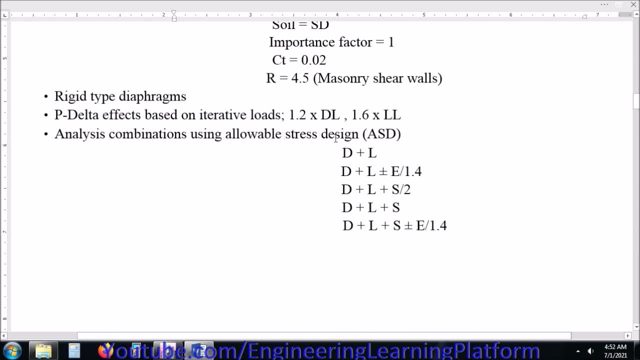 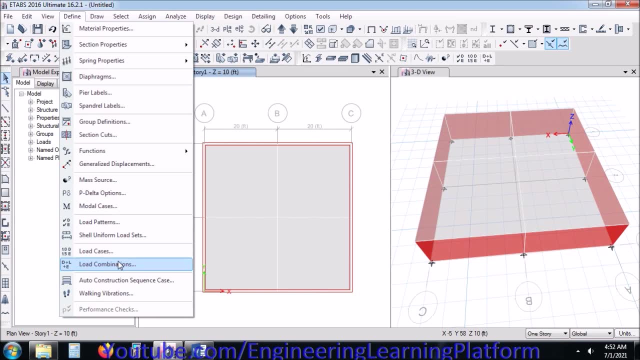 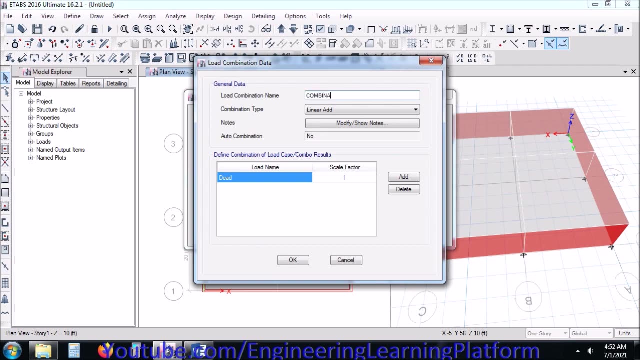 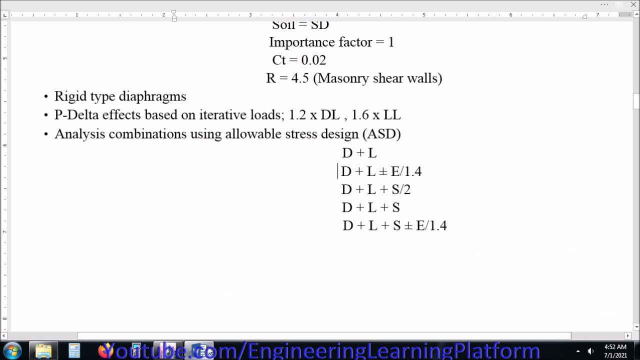 match the slab mashing so that the force transfer becomes accurate. I'll be defining the load combinations simply: dead plus life, that is the service combination and the other dead load is finishes load and click on OK. and now copy the combination and make the earthquake combination, since we are using 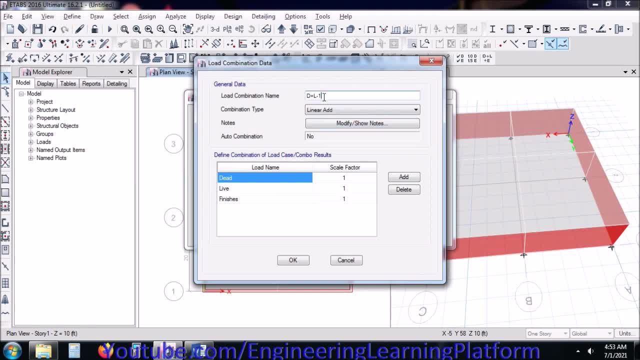 since we will be checking the service stresses as per UBC 97, so we are making these service combinations not ultimate combinations. UBC 97. utilized service combinations for allowable stress design method. machine restructures are designed using allowable stress design method as per previous quotes you. 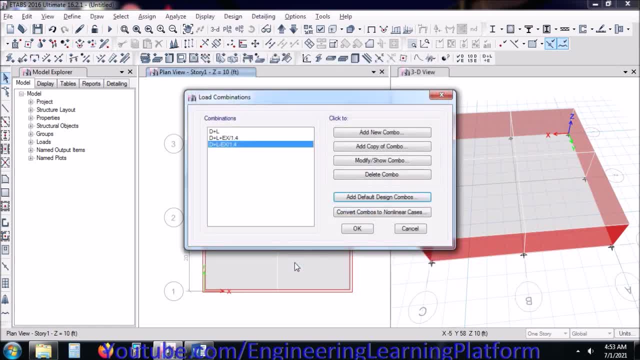 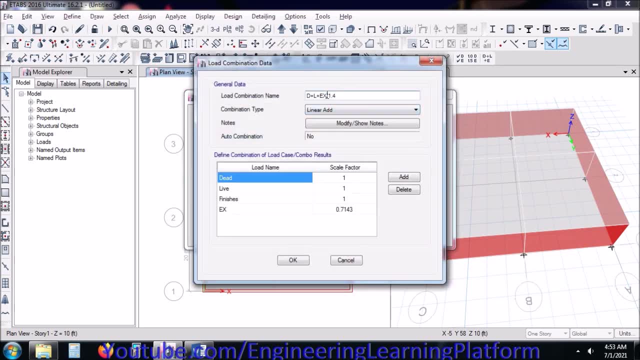 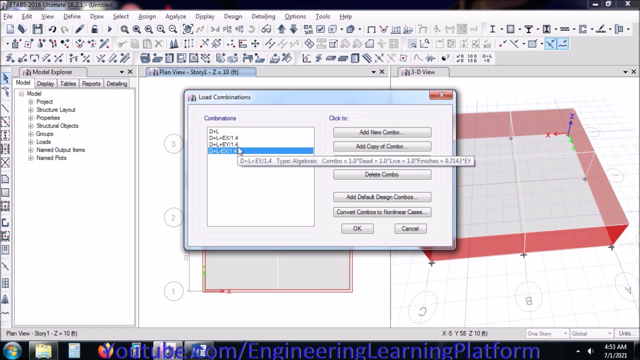 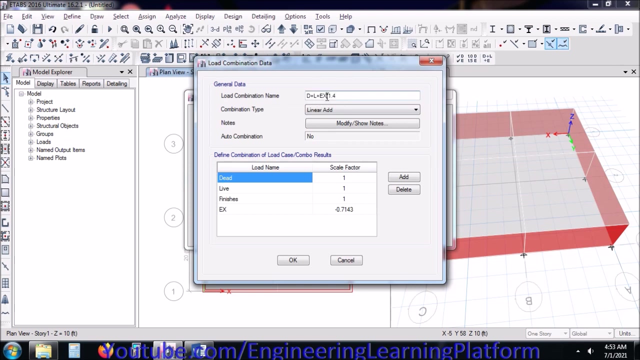 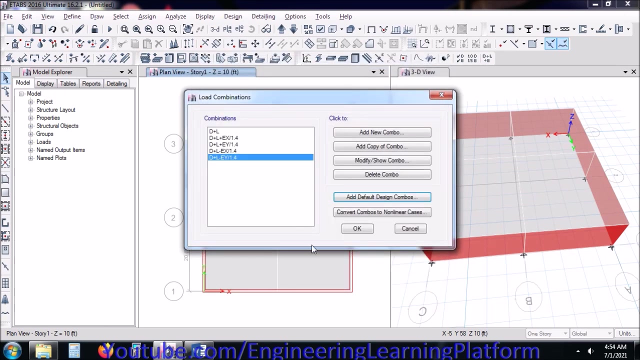 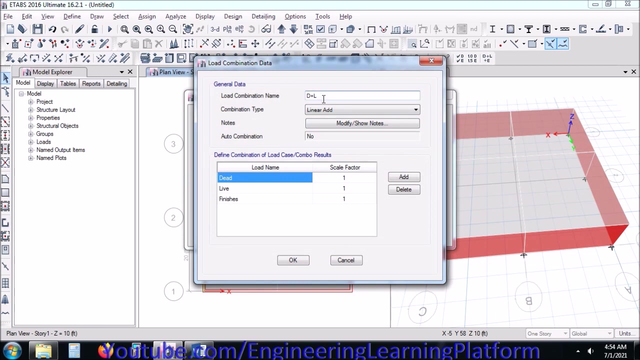 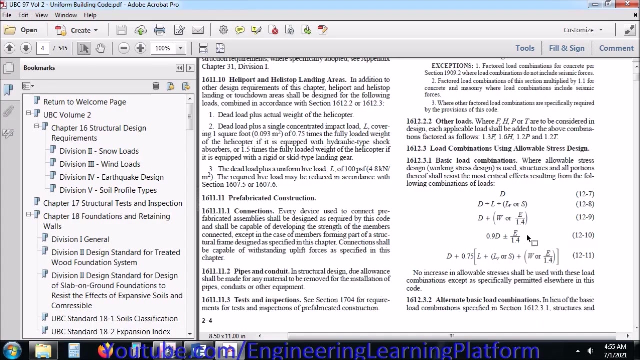 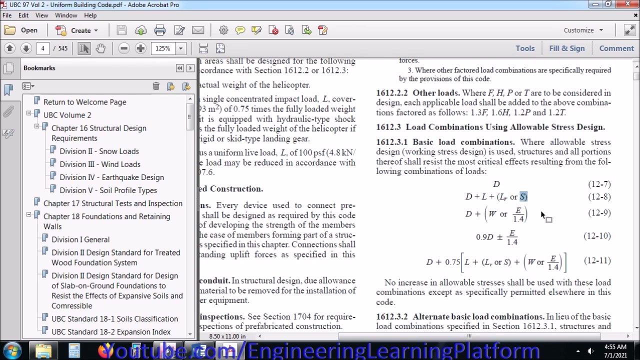 can define the combinations for your chord. now i will be defining the same combination for the y direction, since we have incorporated earthquake in x direction, and load combinations till now, since the shelf load and the snow load are alternatives of each, but here, in our case, the values are both 20psf. the live load for the roof is also 20psf and the live load for 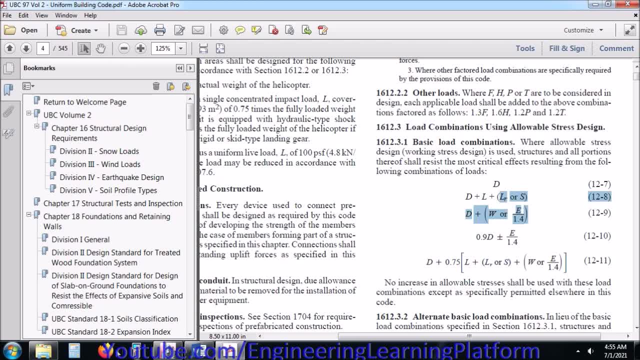 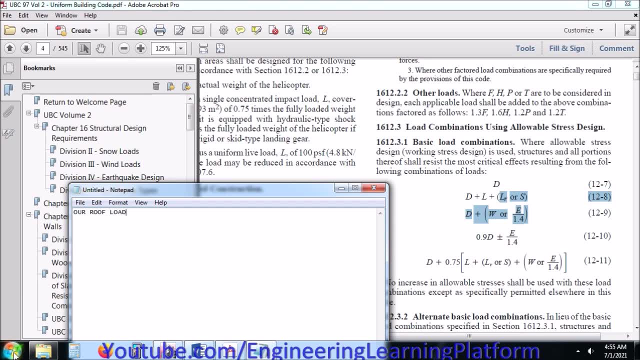 these 20psf snow is also 20 PSF and in combination they are repeating, as so our roof load and the snow load is 20 PSF. that is equal value, so no need to repeat the combination for the snow load, as we have already incorporated the same. 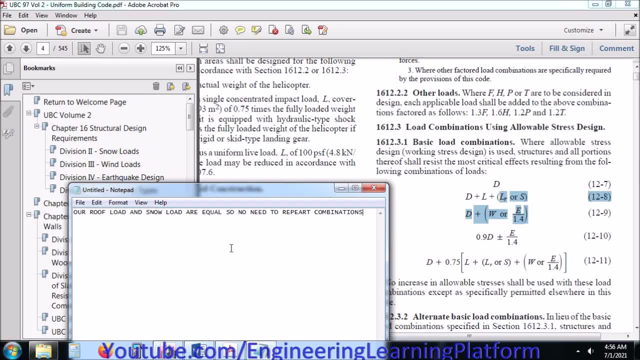 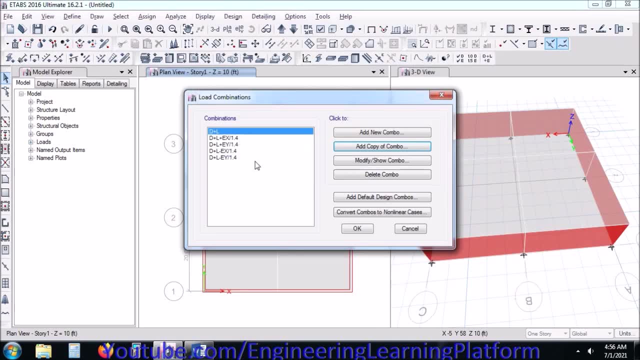 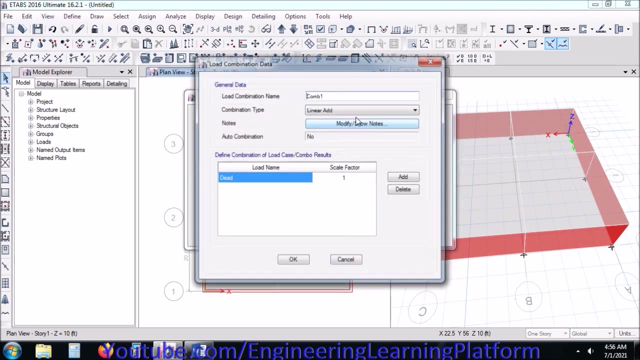 combination for the roof live load. it is a pure coincidence that our roof live load and snow load are same, so I will just keep the thing simple and work with the roof live load only, as the snow load is equal to the live load and the combinations for the snow load and live load are exactly the same as per UBC 97. 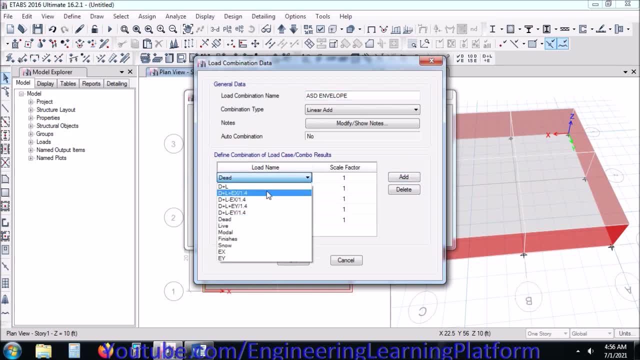 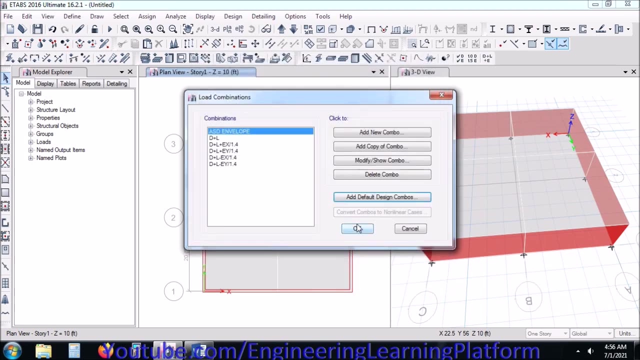 allowable stress design method. if you are using a different code, then you have to see the provisions of the code and control it as well. their combinations: there is no harm if I would have taken the snow load in along with the live load, but just to reduce the efforts and save time. as I know the 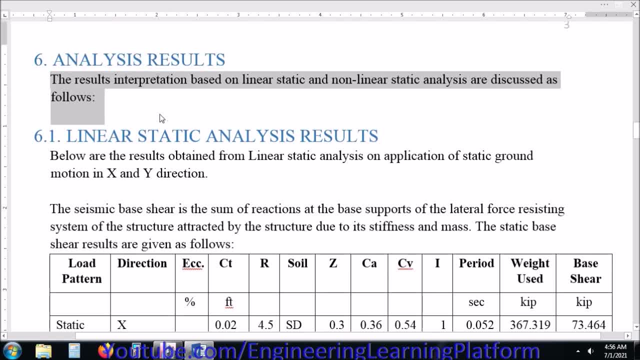 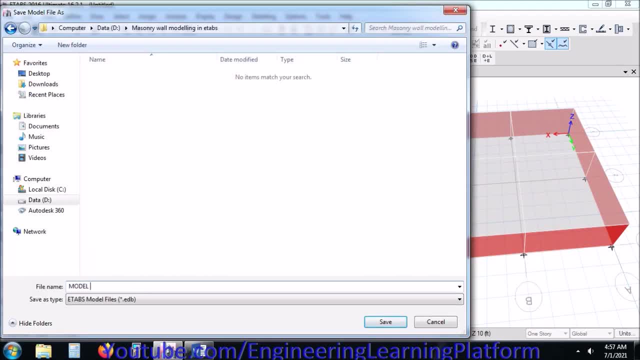 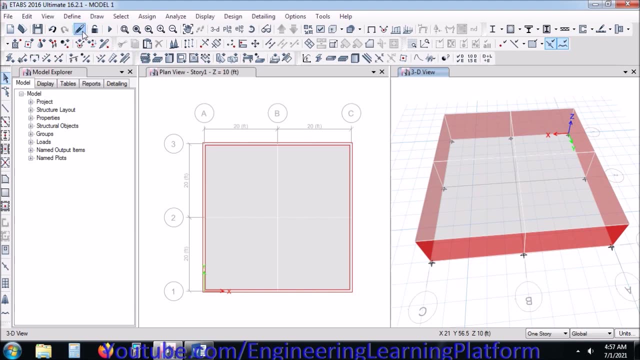 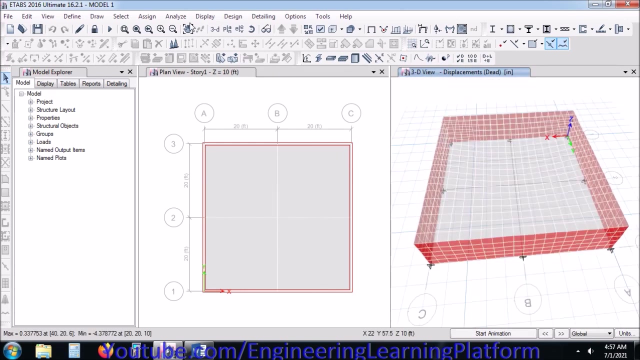 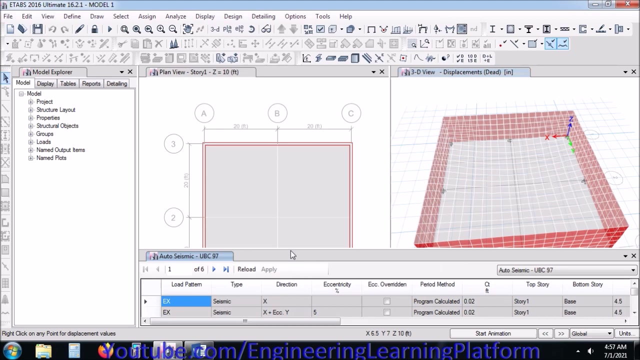 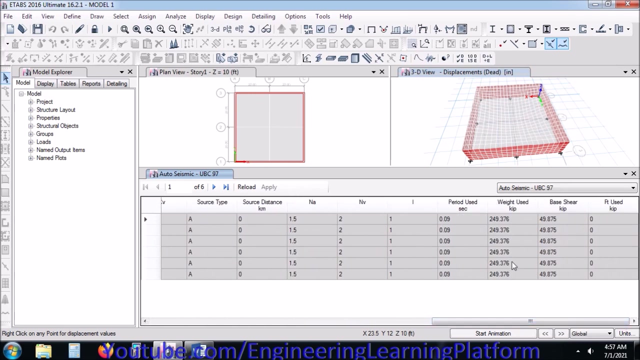 results would be same, so I keep the things unchanged. now let's perform the analysis on the structure. so, if you see, the mesh size is exactly what I wanted, the wall and the slab meshes are exactly matching and the nodes are transferring the loads. let's check the size and base here on the structure, the period and the weight utilized. 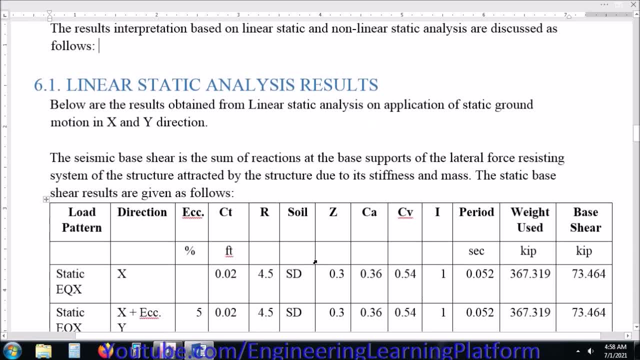 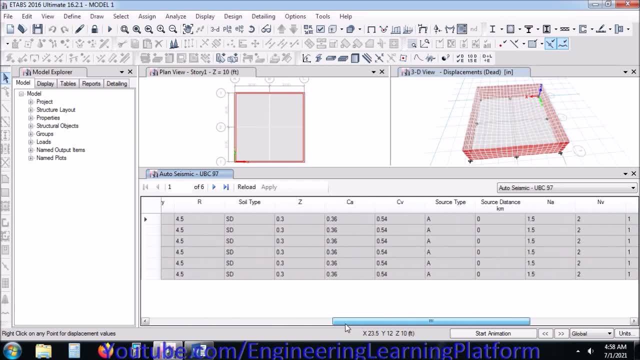 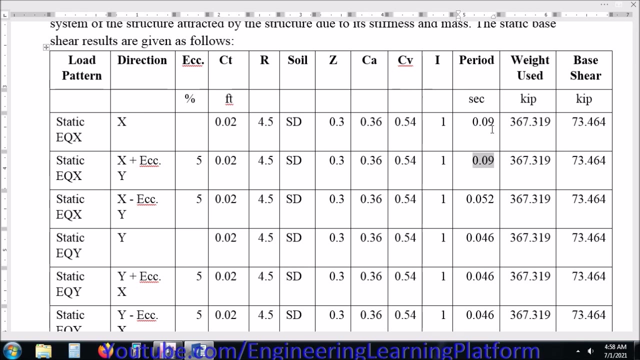 of the structure by eTabs as we define the mass source for the dead loads. only mass votes include dead loads as per UBC 97, and if you want to incorporate live block then structure must be a little bit high-rise. so I'll be editing this list for my project this. 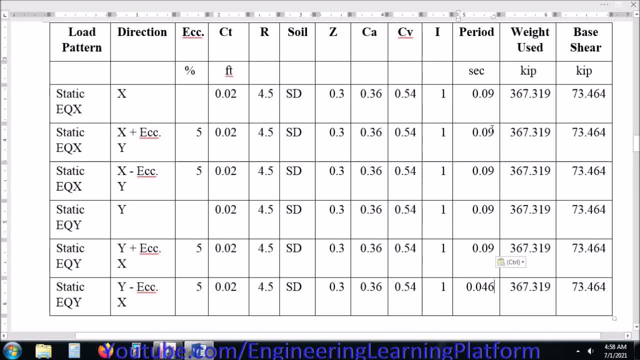 is a related piece and it says chicos. how much would it cost if we file of PERSA, for an example for uk czas? I'm not sure it's the best way to write it. just tell me and I'll recommend the ready-made list and the list's link to download. this document has been attached in description. 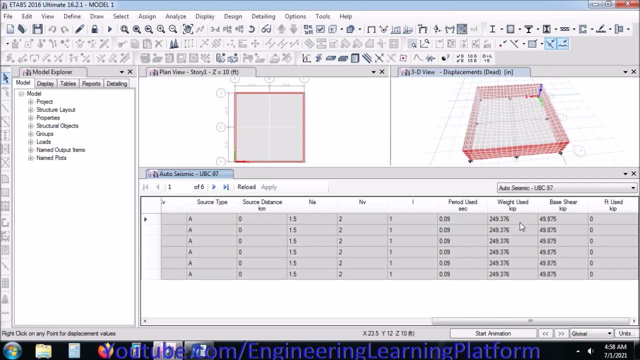 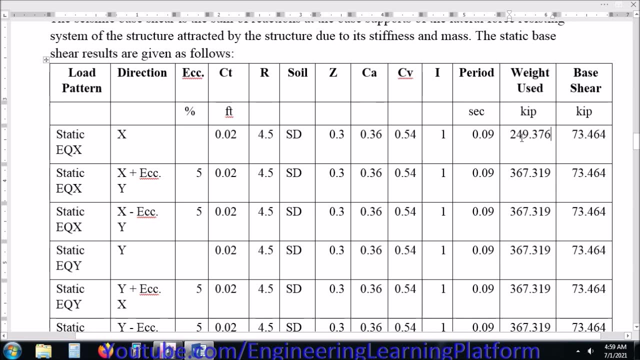 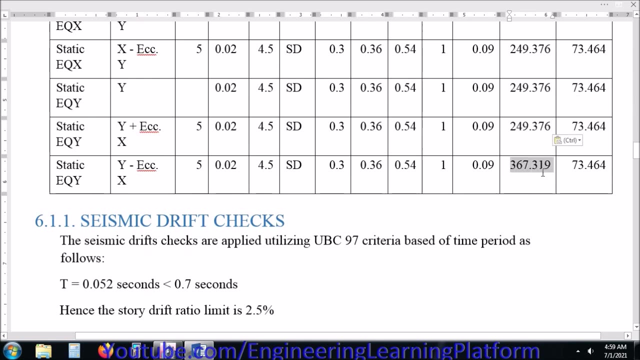 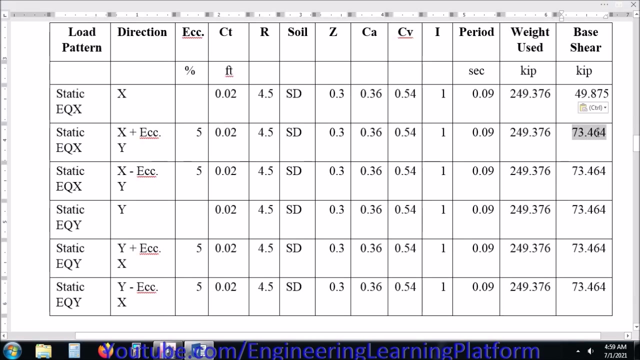 it is a basic masonry structure design report template. you can easily edit these values for your structure and prepare a masonry structure design report in a professional manner. i personally use this report template in my own projects and clients really like it, so you can use the template for your projects as well. link to download this report is given in description. 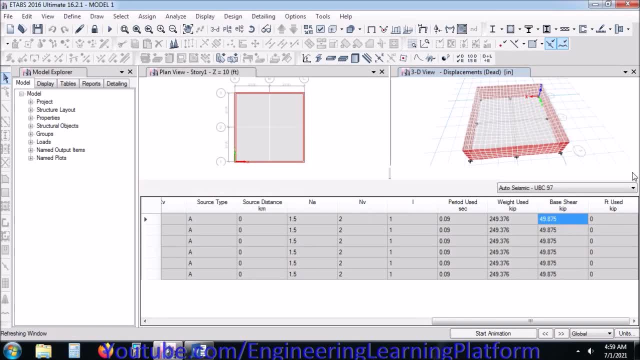 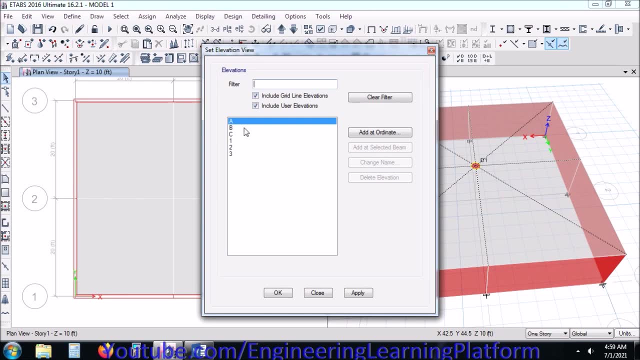 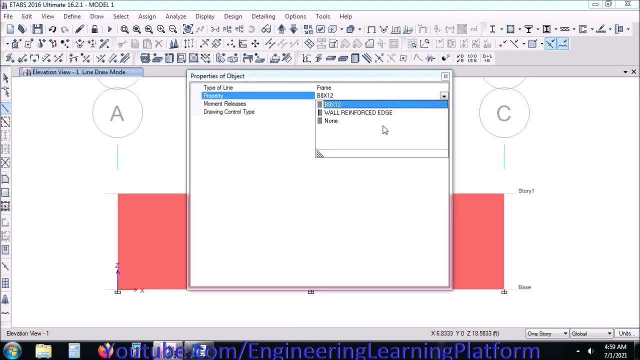 of the video. okay, so i have incorporated the waste weight, utilize of the structure and the base shear, calculated by the software as per the code ubc 97. now let's draw the openings in the walls. actually, we should have drawn the openings in the walls, you. 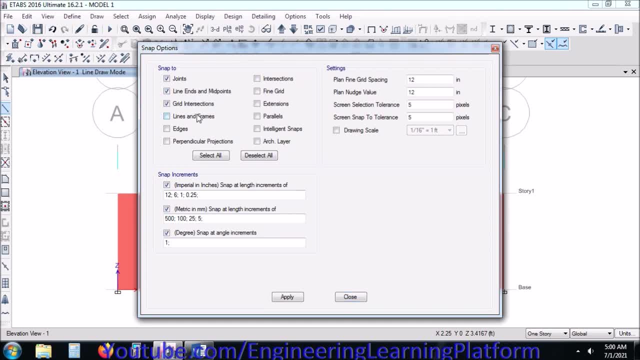 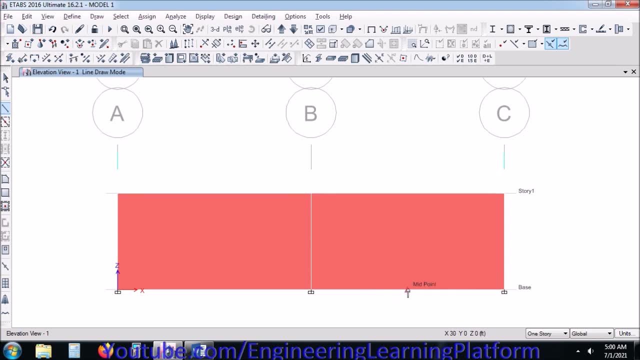 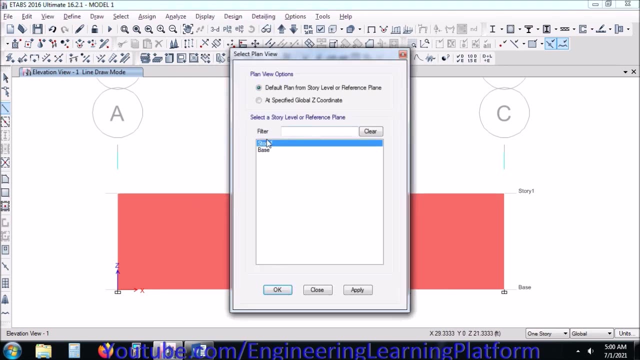 and completed the model in a previous stage. but let's just try to do it, as i just have to see that the model we have done so far is right and for demonstration purposes. the structural behavior will not change much, as it's a masonry structure. so if we add openings, 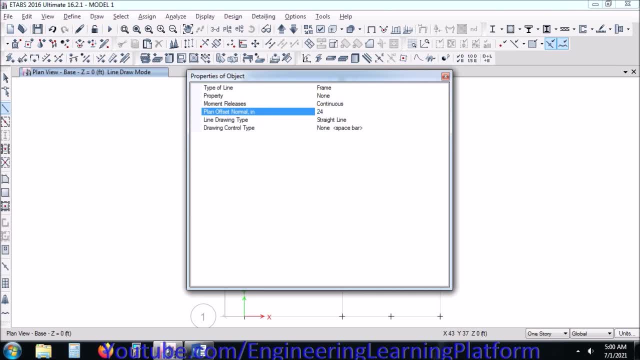 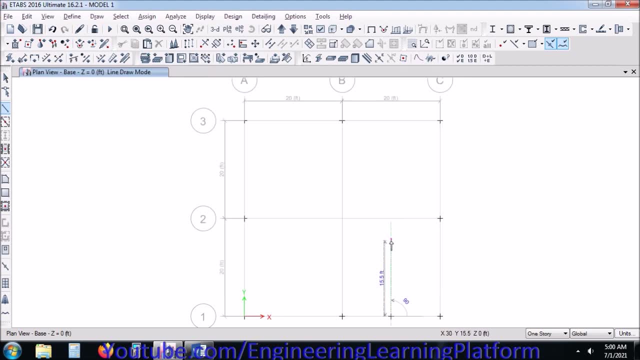 along with the lintel and the spandrel, and the die beams along with the band beams. so the behavior of the structure will not change much. however, the stresses in the structure will reduce the more corner elements we add. so i'm creating a doorway in the wall. 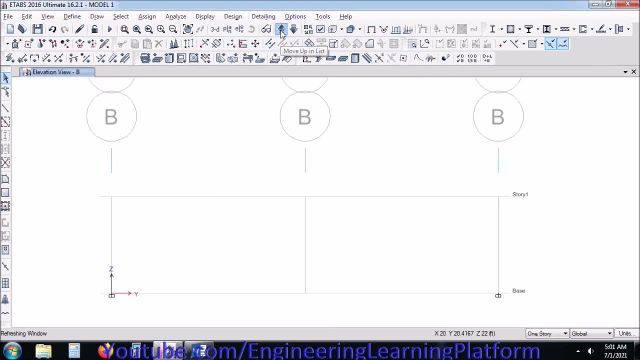 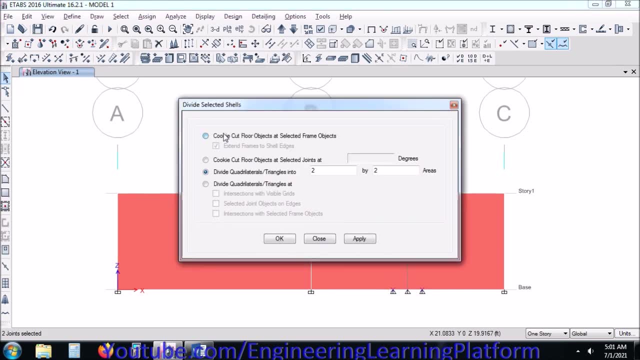 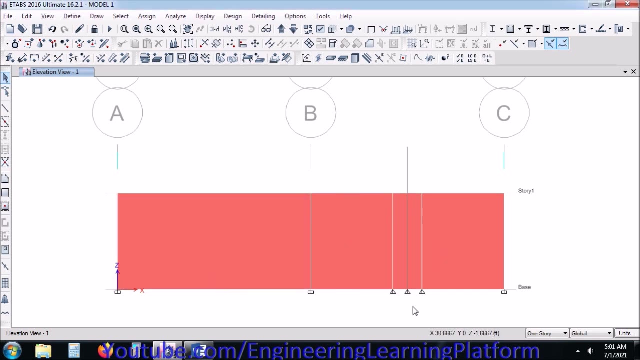 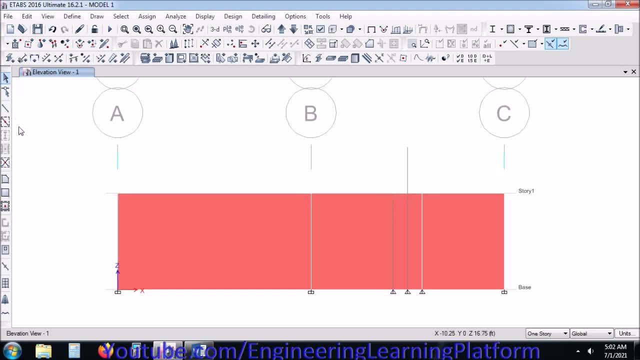 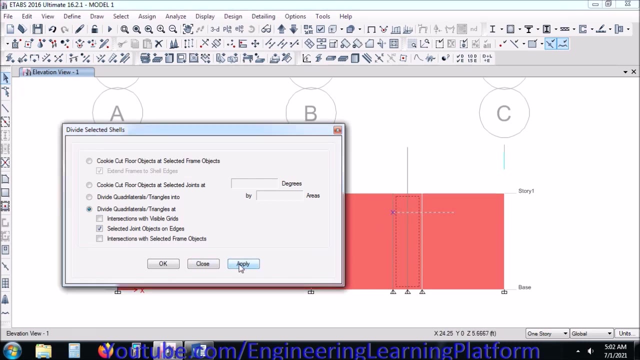 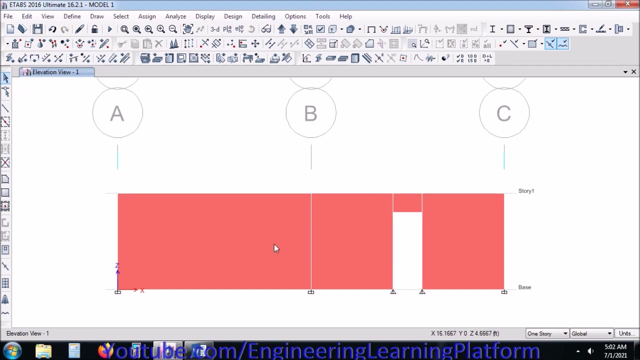 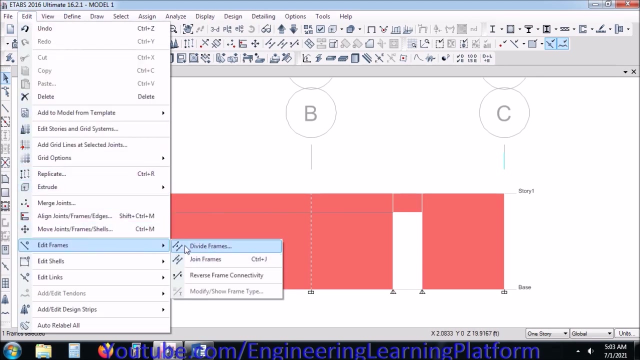 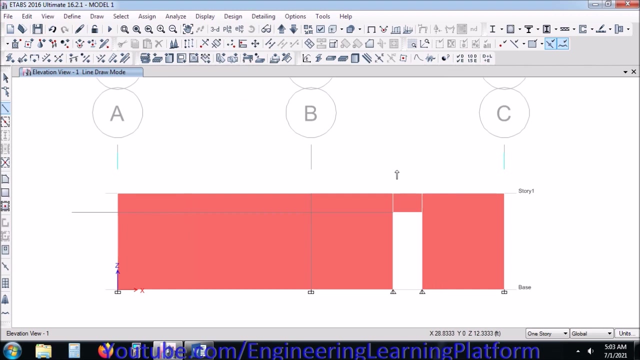 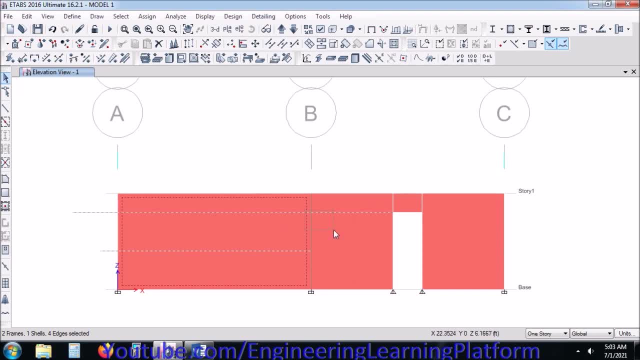 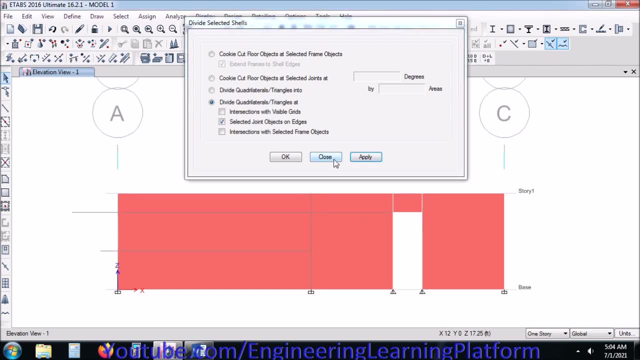 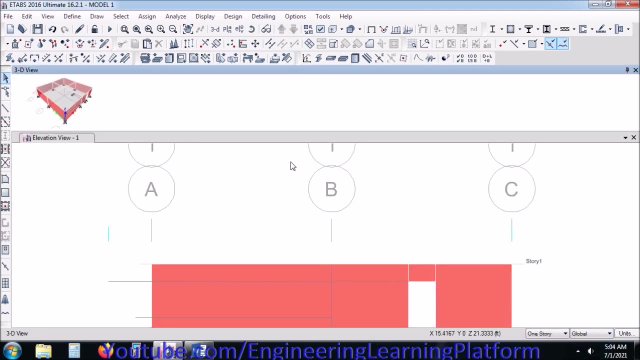 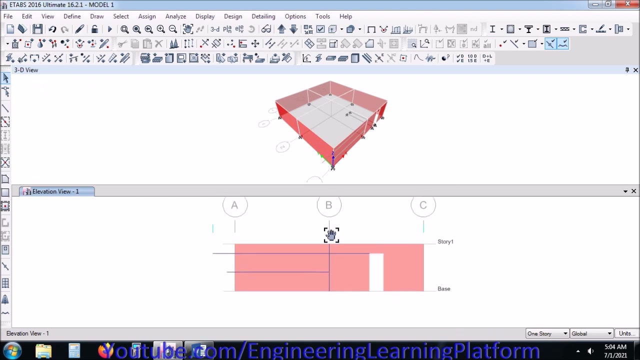 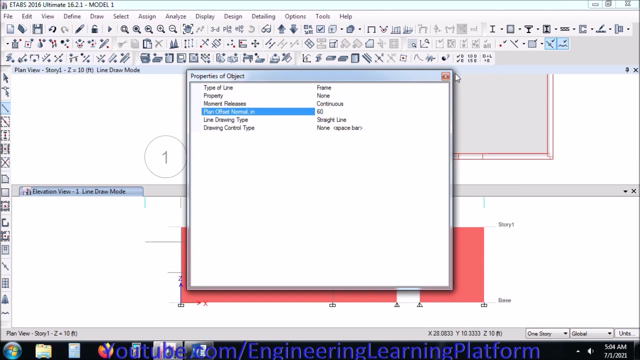 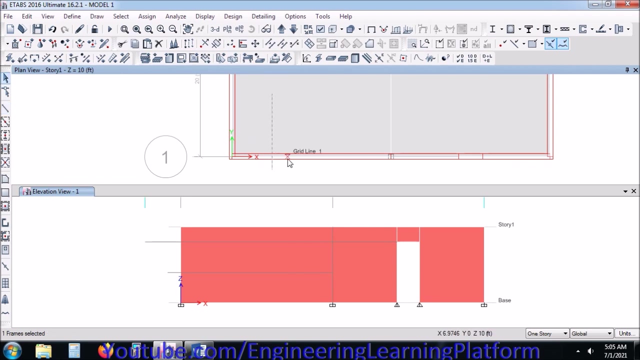 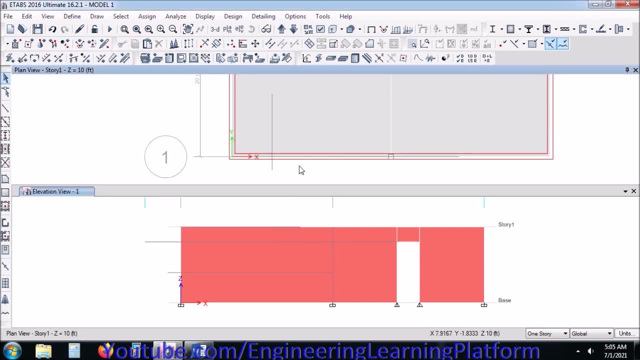 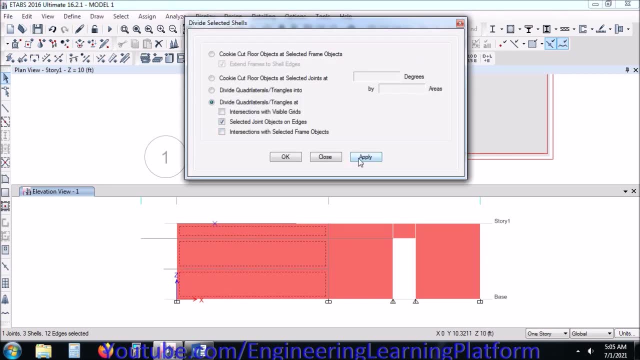 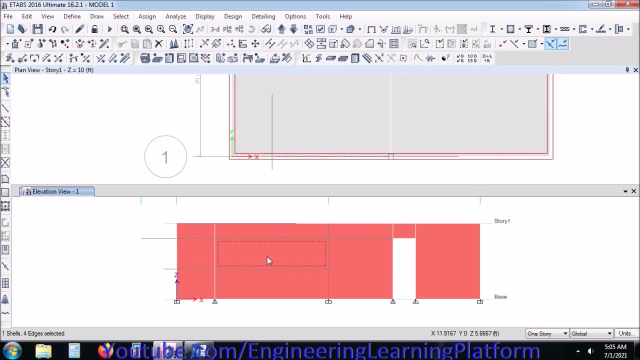 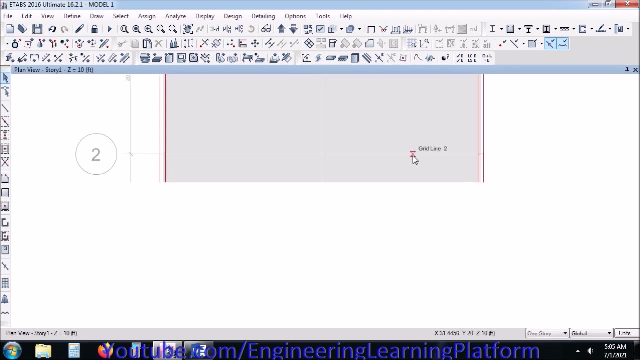 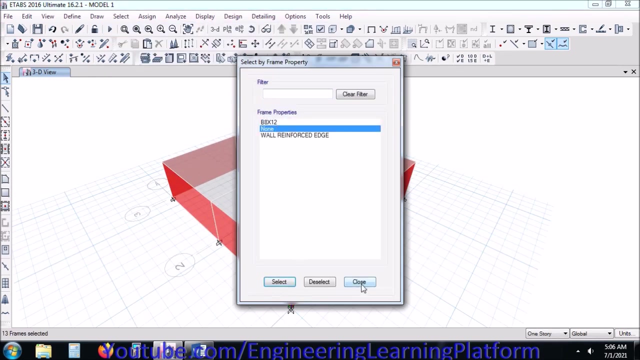 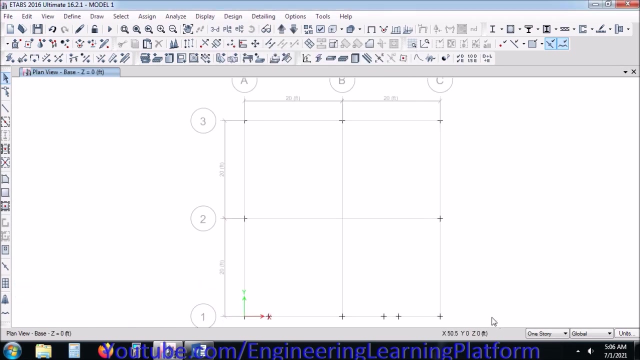 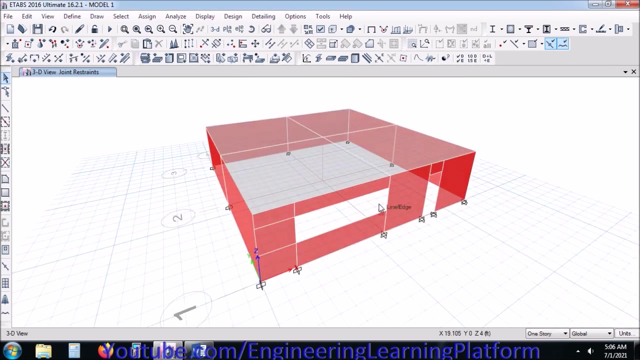 so. so i have made the window opening here. so after assigning the openings in the masonry structure, we will be checking the preliminary. so after assigning the preliminary, so after assigning the preliminary stresses in the structure. so i've made these supports as fixed and save the model. 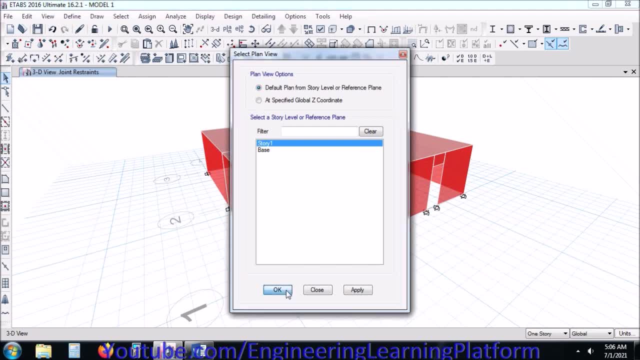 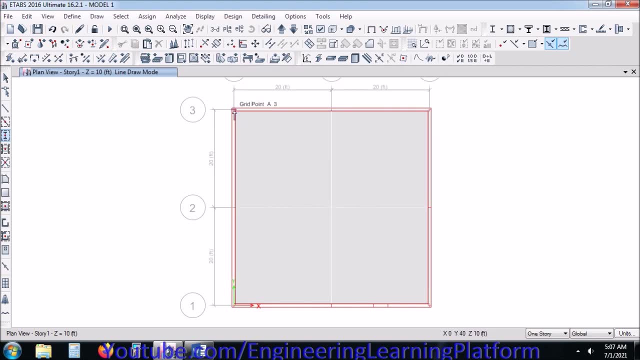 and save the model. now i'll be assigning the corner elements. now i'll be assigning the corner elements. now i'll be assigning the corner elements of the walls, of the walls, of the walls, that is, the reinforced concrete edges and the band beams, of course, and the band beams, of course. 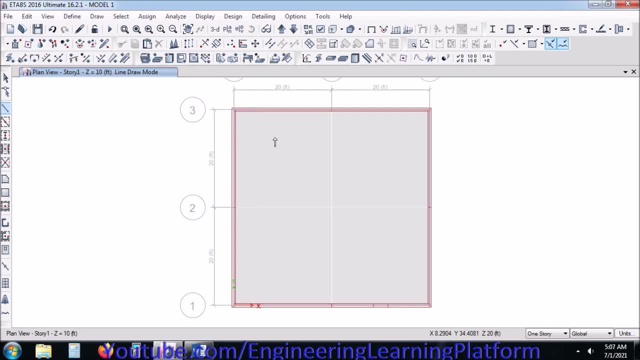 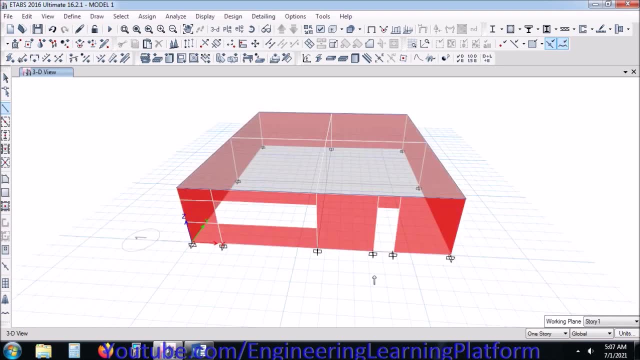 and the band beams, of course. so the band beam will come just beneath, so the band beam will come just beneath. so the band beam will come just beneath the slab and it will perform as a. and it will perform as a and it will perform as a bonding agent between the. 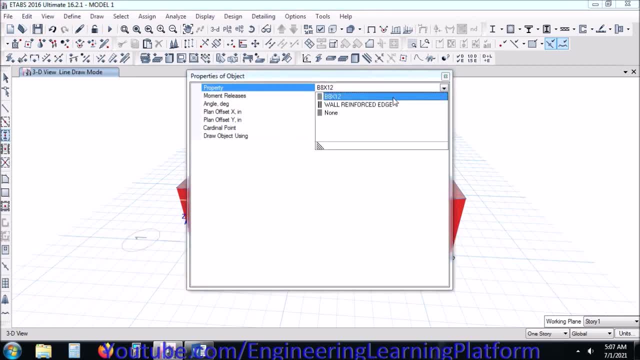 bonding agent between the bonding agent, between the wall and the reinforced concrete slab wall and the reinforced concrete slab wall and the reinforced concrete slab, and it will form joint with the and it will form joint with the and it will form joint with the reinforced concrete. reinforced concrete. 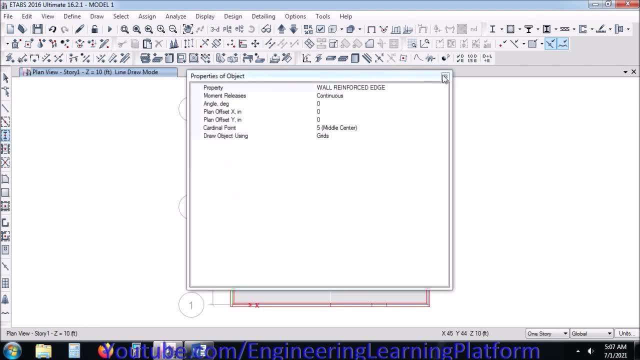 reinforced concrete edges of the wall which i will be placing, edges of the wall which i will be placing, edges of the wall which i will be placing right now, right now, right now. so this is the reinforced concrete edge. so this is the reinforced concrete edge, so this is the reinforced concrete edge which we define. 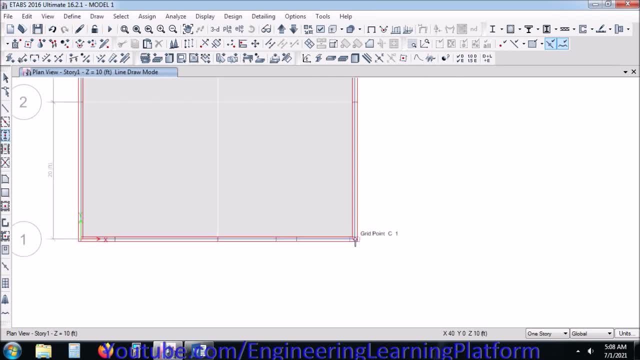 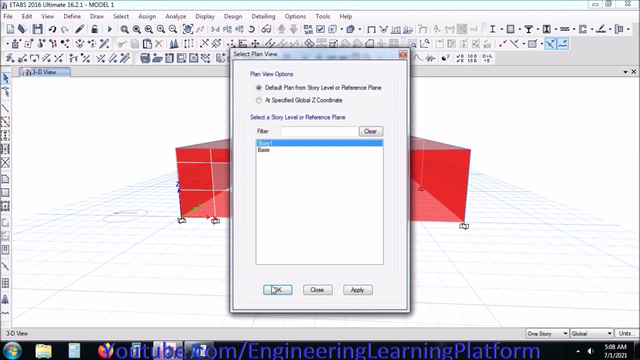 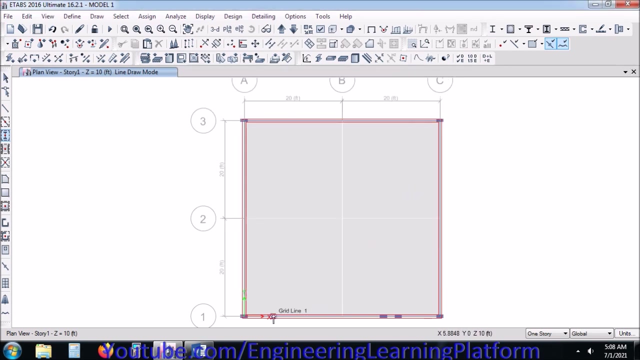 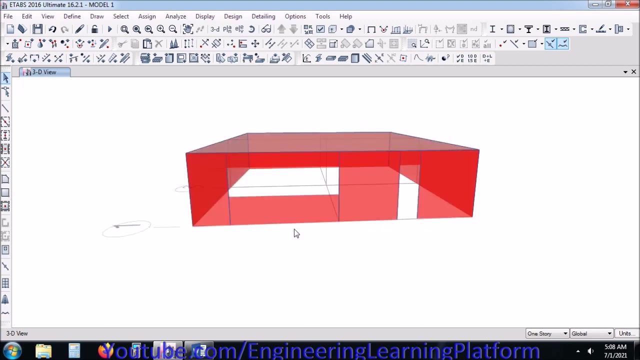 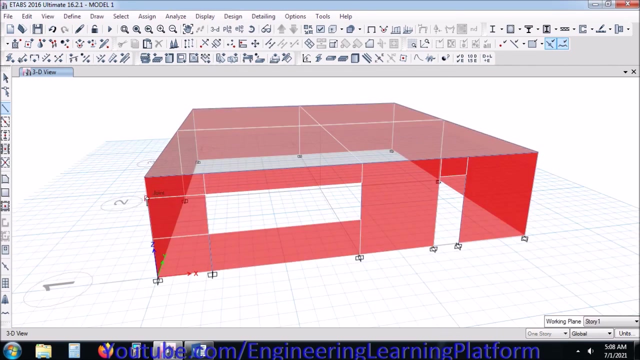 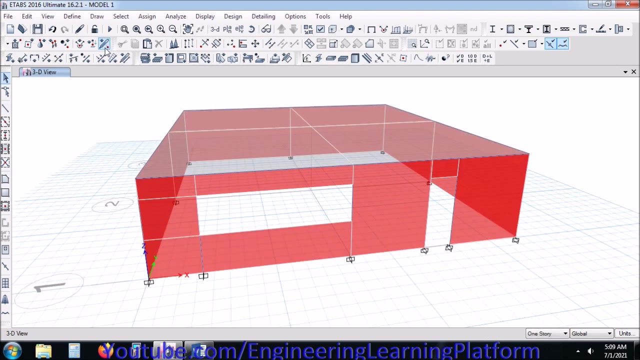 which we define, which we define just like a column, just like a column, just like a column. right now, we haven't added the internal. right now, we haven't added the internal. right now, we haven't added the internal partition wall, partition wall, partition wall in the structure. we will be checking. 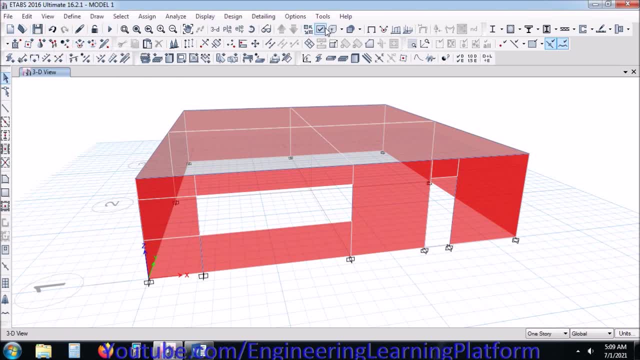 in the structure. we will be checking in the structure, we will be checking the results of these stresses, the results of these stresses, the results of these stresses in the next part of this lecture, in the next part of this lecture, in the next part of this lecture and the link to the next part of the. 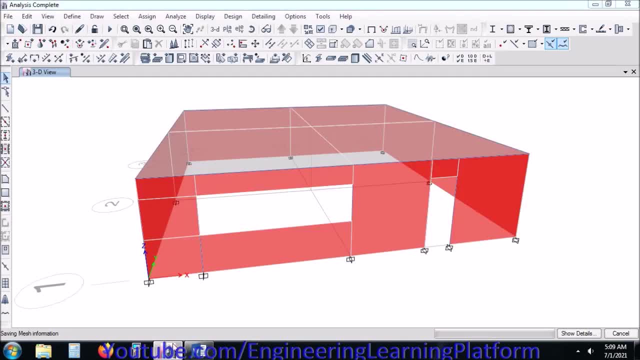 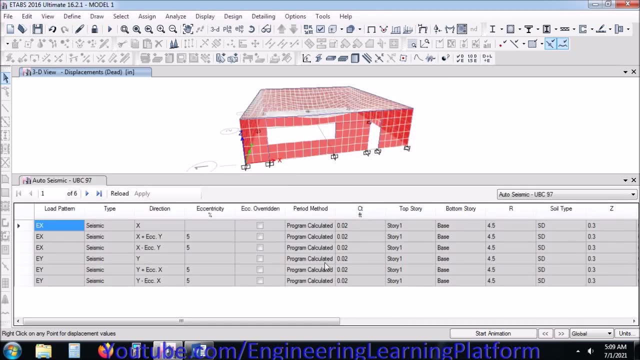 and the link to the next part of the and the link to the next part of the lecture is given in lecture is given in lecture is given in description of this video. however, we can check the seismic base. however. we can check the seismic base. however, we can check the seismic base here again and see if there is any much. 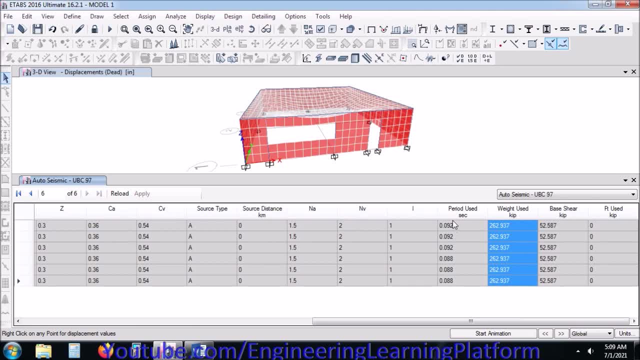 here again and see if there is any much here again and see if there is any much difference, and then we'll be adding the interior, and then we'll be adding the interior and then we'll be adding the interior. partition, partition partition, walls in the structure, walls in the structure. 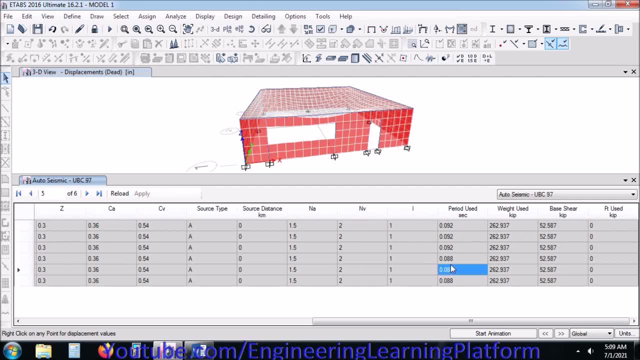 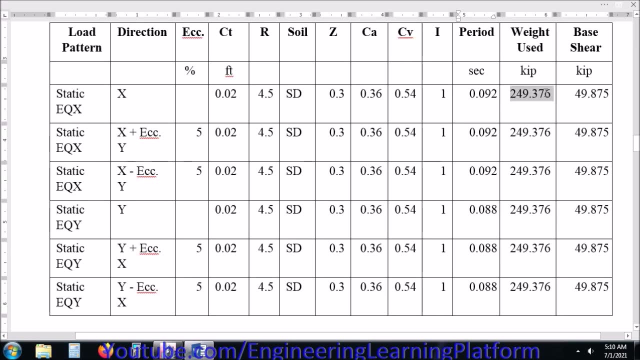 walls in the structure, as the spans according to, as the spans according to, as the spans according to the first, the first, the first modeling, modeling, modeling. the spans are quite large for a, the spans are quite large for a. the spans are quite large for a masonry structure. so there are large. 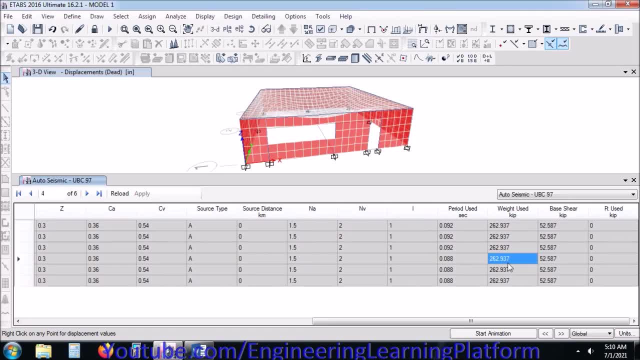 masonry structure. so there are large masonry structure, so there are large deformations in the slab and large force deformations in the slab and large force deformations in the slab and large force transfer from the transfer, from the transfer from the slab to the walls. so definitely the 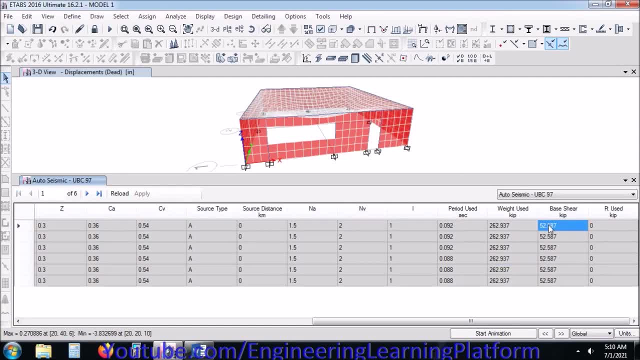 slab to the walls, so definitely the slab to the walls, so definitely the stresses in the walls will be exceeding, stresses in the walls will be exceeding stresses in the walls will be exceeding, which we will check in the next part, which we will check in the next part. 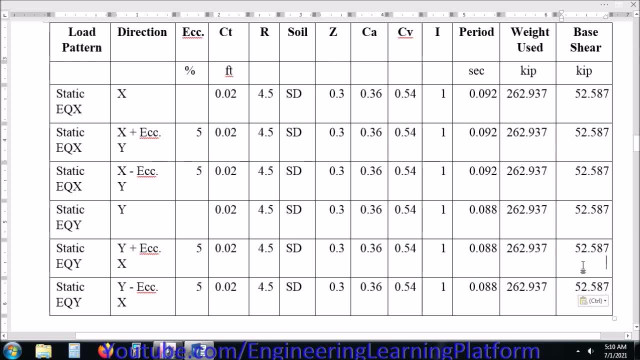 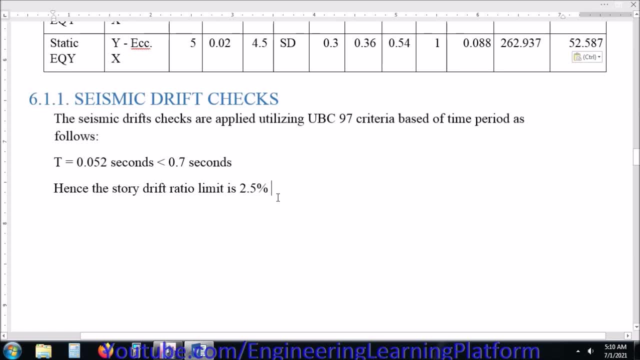 which we will check in the next part. similarly, we will perform the checks for. similarly, we will perform the checks for. similarly, we will perform the checks for seismic drift. and you can download this report template. you can download this report template. you can download this report template. the link to download. 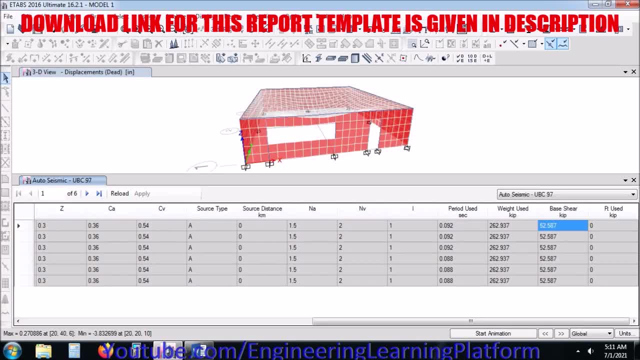 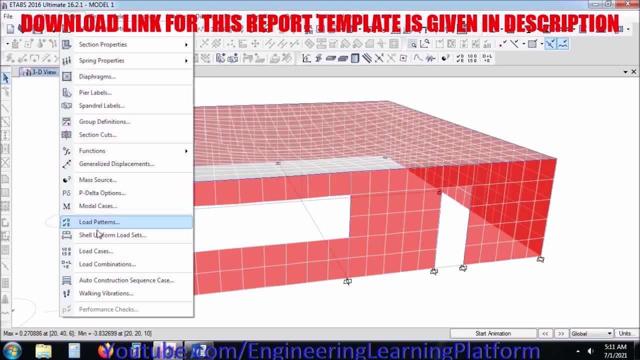 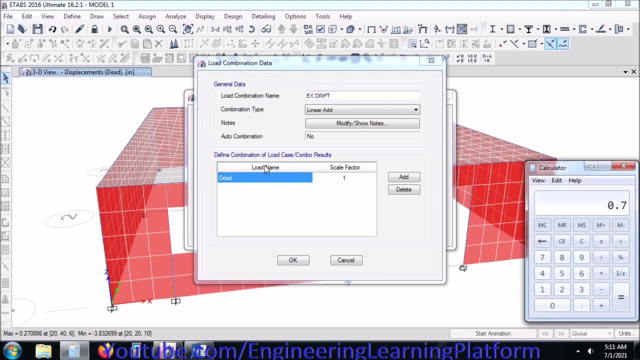 let's define the load combination of the. let's define the load combination of the envelope envelope envelope and the earthquake drifts and the earthquake drifts and the earthquake drifts. since we are using ubc 97, the drift. since we are using ubc 97, the drift. 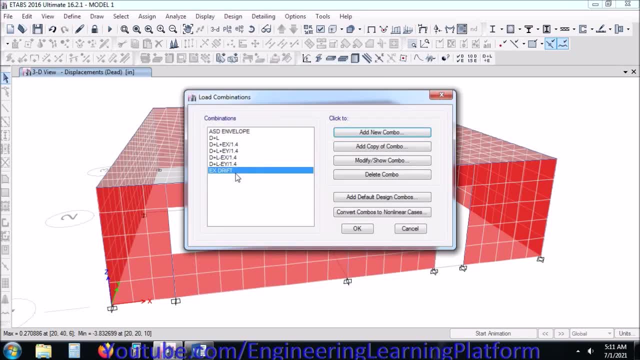 since we are using ubc 97, the drift, the drift. the drift is 0.7, is 0.7 is 0.7 into strength reduction factor times. the into strength reduction factor times. the into strength reduction factor times. the elastic drift, elastic drift. 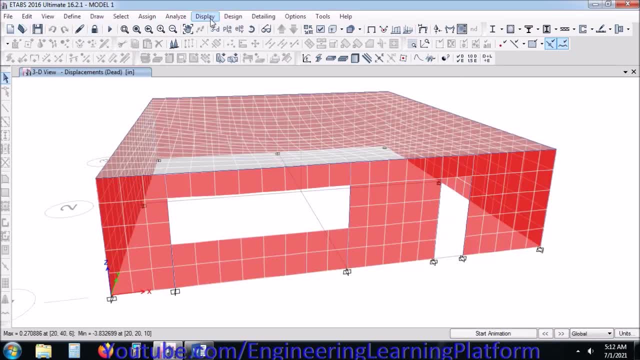 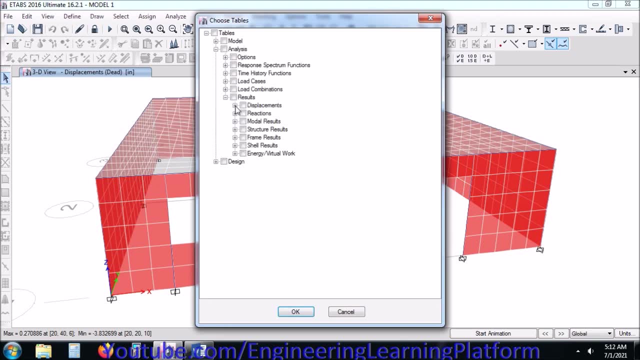 elastic drift: the seismic base shear is elastic. the seismic base shear is elastic. elastic drift: the seismic base shear is elastic. so we have to increase it by 0.7. so we have to increase it by 0.7. so we have to increase it by 0.7 r times. you can use the drift criteria of 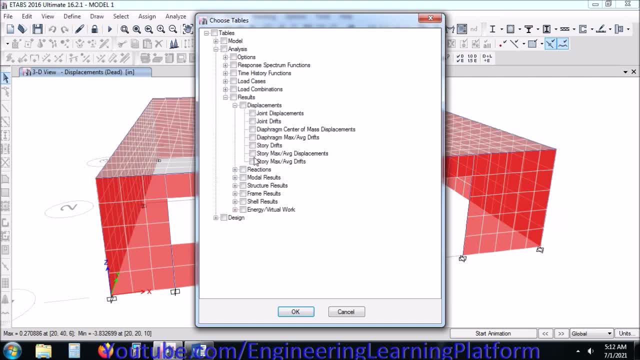 r times. you can use the drift criteria of r times. you can use the drift criteria of your respective code. now. we'll have to click here: add story. now. we'll have to click here: add story. now. we'll have to click here: add story. maximum or average displacements and. 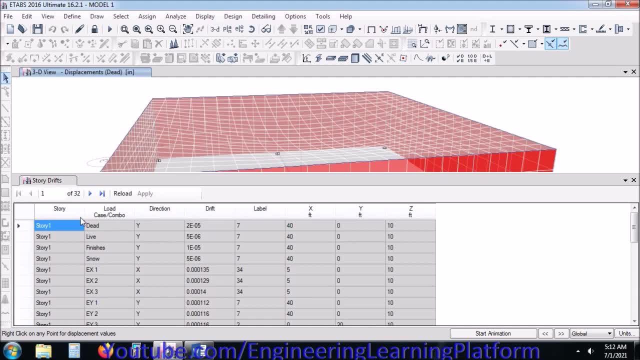 maximum or average displacements and maximum or average displacements, and check it with our, check it with our, check it with our code criteria, code criteria, code criteria, since we are checking drift, for since we are checking drift, for since we are checking drift for earthquake, load only. 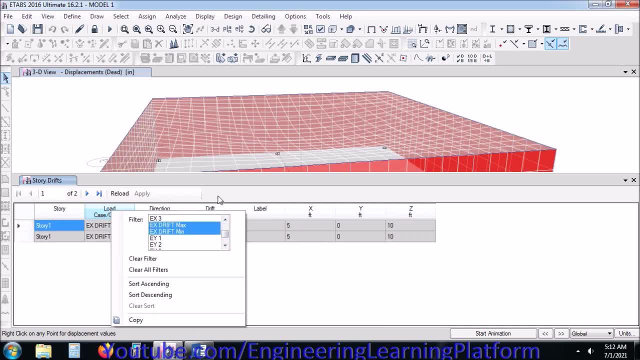 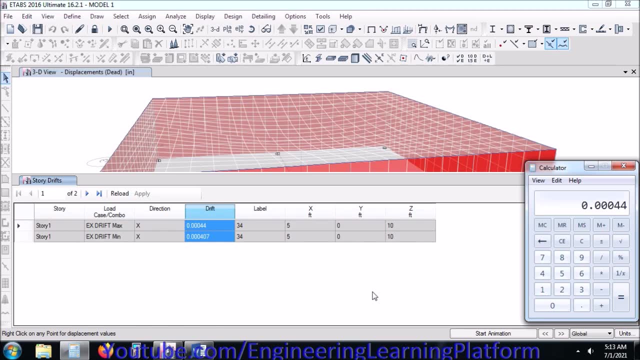 earthquake load only. earthquake load only. earthquake drift: maximum and minimum. earthquake drift: maximum and minimum. earthquake drift maximum and minimum. the drift limit as per ubc 97 is the drift limit. as per ubc 97 is the drift limit. as per ubc 97 is two percent. 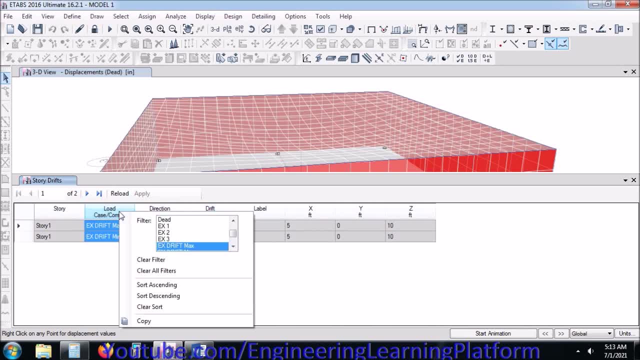 two percent, two percent or 2.5 percent because the time period is, or 2.5 percent because the time period is, or 2.5 percent because the time period is less than 0.7 seconds. less than 0.7 seconds. 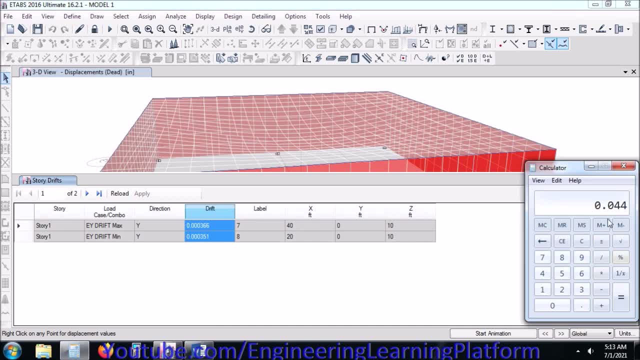 less than 0.7 seconds. so we are okay in x direction, now let's. so we are okay in x direction, now let's. so we are okay in x direction. now let's check for the y direction. check for the y direction. check for the y direction. in percentage, it is 0.36 percent, which is